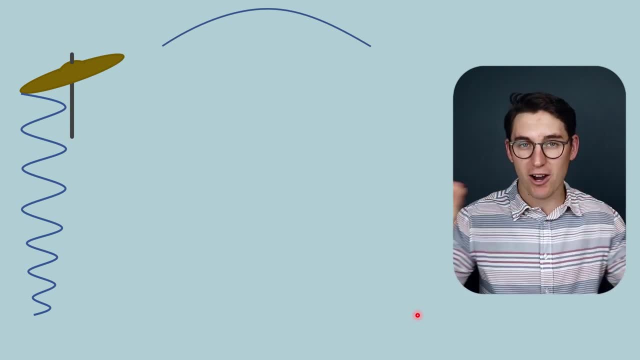 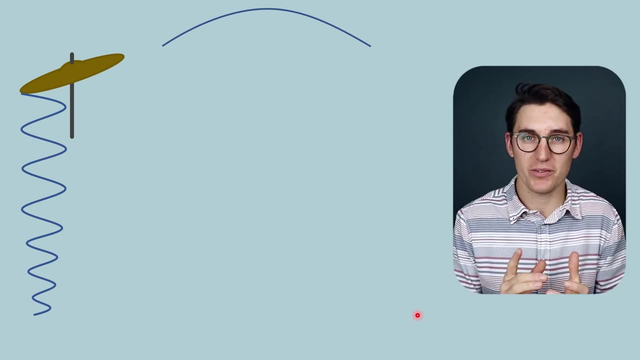 it will resonate at a certain frequency depending on how far those set points are apart and how taut that string is, much like the width of our piezoelectric material. Now, in all of these cases, the resonance will happen at a specific frequency based on the characteristics of the instrument or 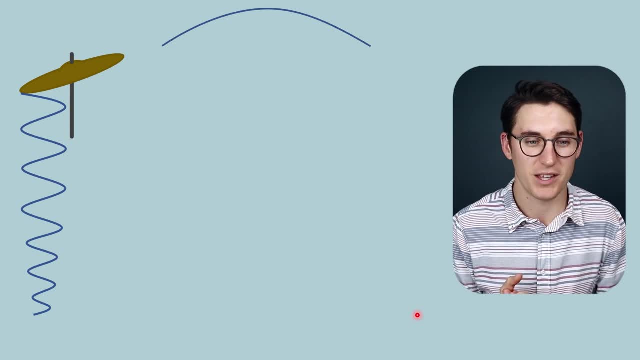 the piezoelectric material that is creating that resonance frequency. This frequency that we transmit into the tissues is what's known as the fundamental frequency, based on the thickness of our piezoelectric material. So if we had a look at a guitar string, 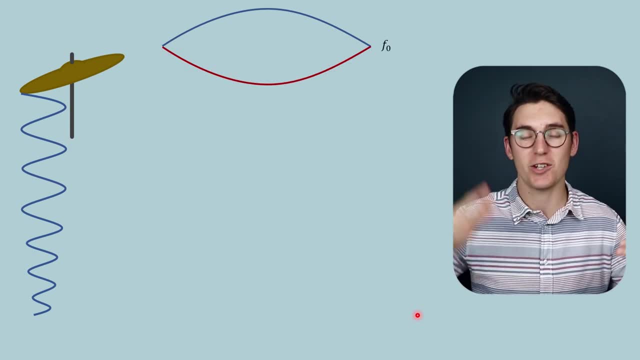 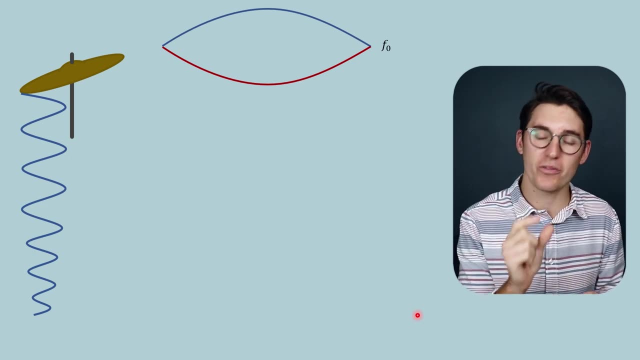 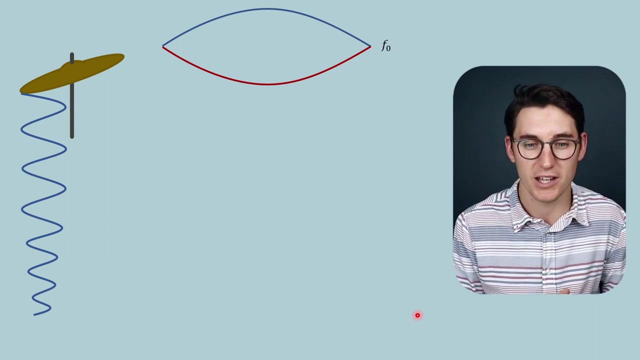 and we pluck a guitar string, we get this half wavelength standing wave resonating at our fundamental frequency. Now, a harmonic frequency is an integer multiple of this resonance frequency. What does an integer multiple mean? It means it's a whole number multiple of this frequency. So if this was resonating at 2 MHz, 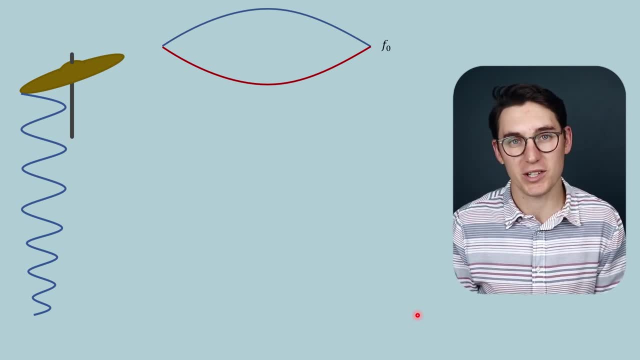 resonating at 2 megahertz. the first multiple integer that we can get is 4 megahertz. We times this base resonance frequency by 2. We can then times it by 3,- we get 6 megahertz. Times it by 4, get 8 megahertz, And what we can see is that 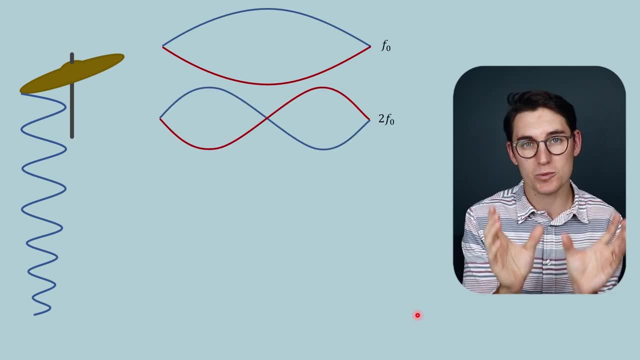 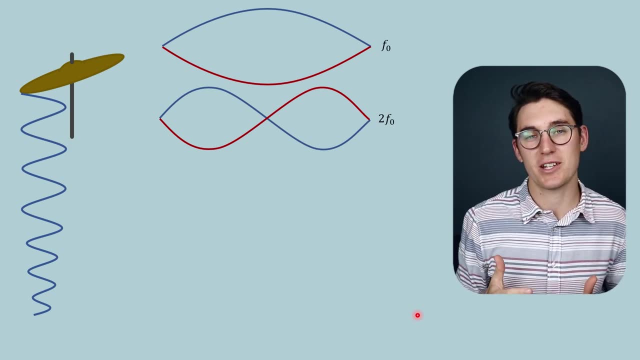 this fundamental frequency can be separated into smaller harmonic frequencies. Now, when a wave interacts with tissues, the echo returning will be the same as the fundamental frequency And there are a couple of reasons now that we're going to look at that will also get returning echoes coming in. 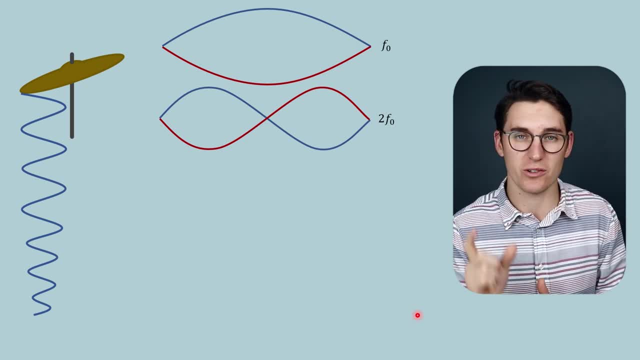 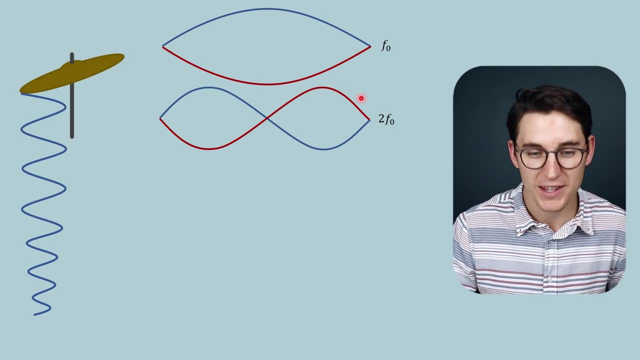 these harmonic frequencies integer multiples of that original fundamental frequency. So here we can see we've got a frequency that's double that of our fundamental frequency. This is our first harmonic, or two times our fundamental frequency. And these regions where the wave is still, these are what's known as. 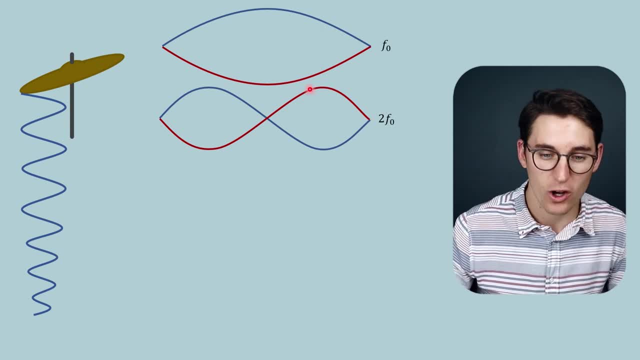 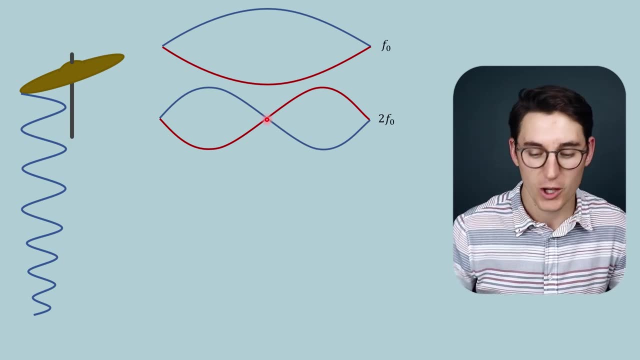 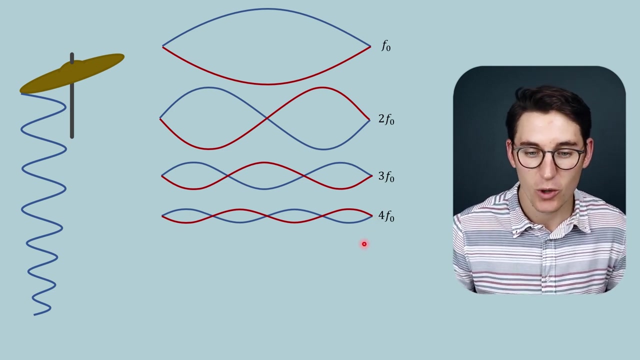 the nodes And the waves moving up and down like this are called standing waves. They will resonate maintaining the shape. here This node will be a point that doesn't move on the wave. We can then get second and third order harmonics, which represent three and four times the fundamental frequencies We 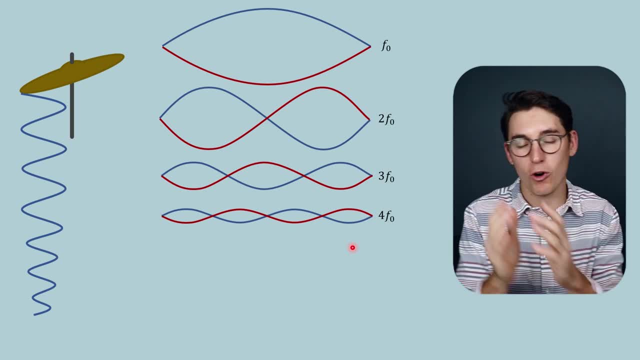 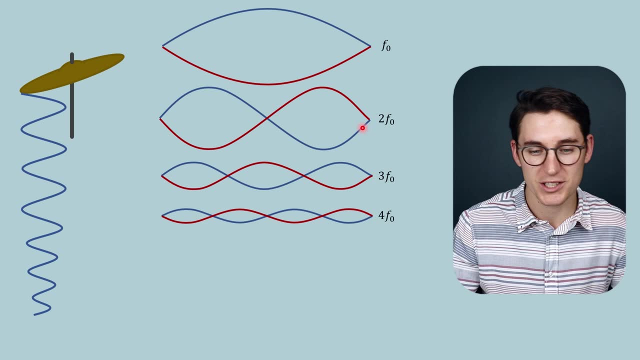 can't get two and a half times the fundamental frequencies. It has to be a whole number, an integer of that original fundamental frequency. So these waves, these higher frequencies, are what is known as the harmonic frequencies and they're based on this fundamental frequency. Now, when we're looking at a 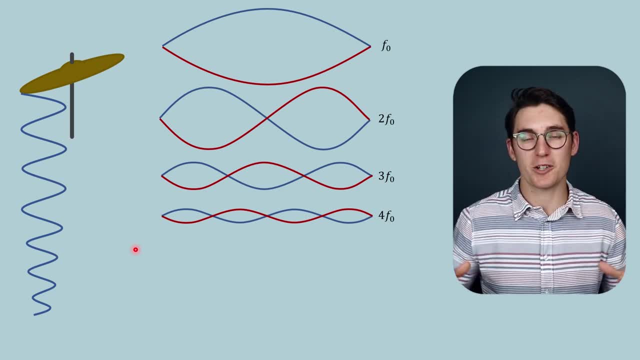 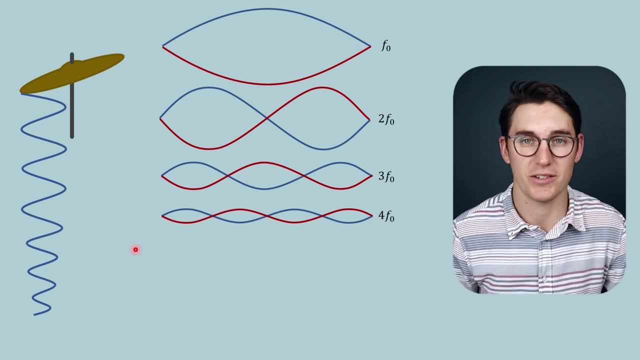 wave like this. we're looking at a one-dimensional wave. It's only got magnitude, It's got frequency, It doesn't have direction and it is not moving through time and space. These are standing waves. here. Now we can get fundamental and harmonic frequencies. 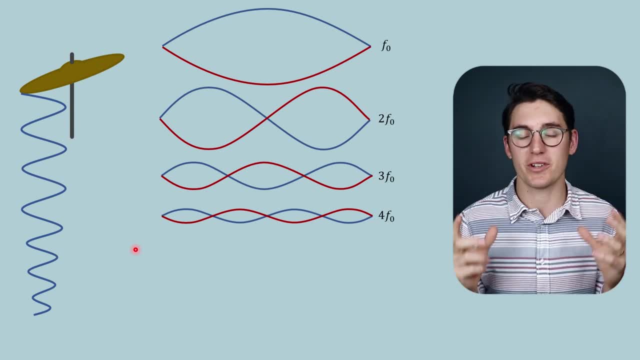 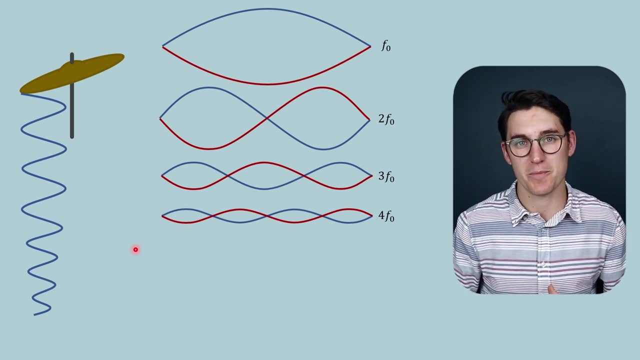 in the two-dimensional realm as well. Now, this is a little bit more difficult to conceptualize and there are some videos on YouTube that you can go and search, where people have made a speaker and placed sand on top of that speaker And when a specific note is played. a. 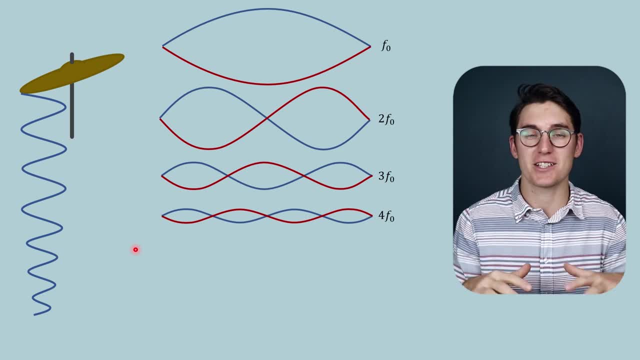 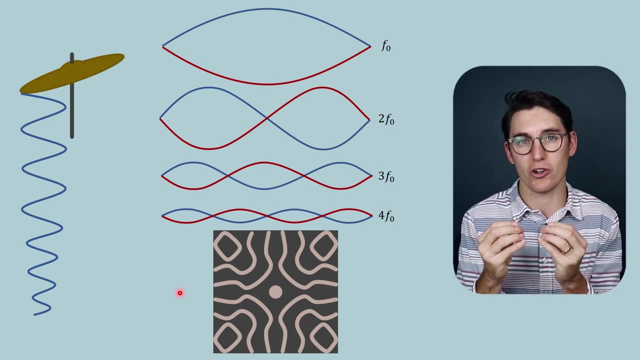 certain frequency is played, the sand will make specific patterns on top of that speaker. So I've drawn a diagram here. You think of this as the top of the speaker here and we're playing a specific note. The speaker is resonating at a specific frequency. You can see that. 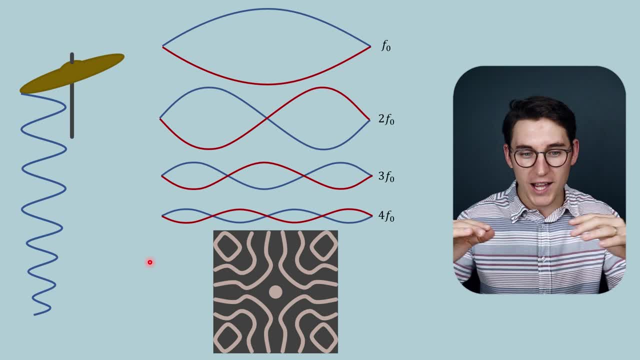 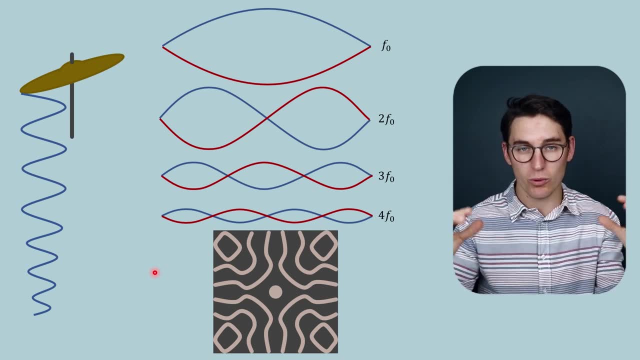 the sand represented by these light lines here will fall down to the nodes on those standing waves. The parts of the speaker that aren't moving the sand because of gravity will fall into those regions and will make a specific pattern. here This is representing the two-dimensional harmonic frequencies. If 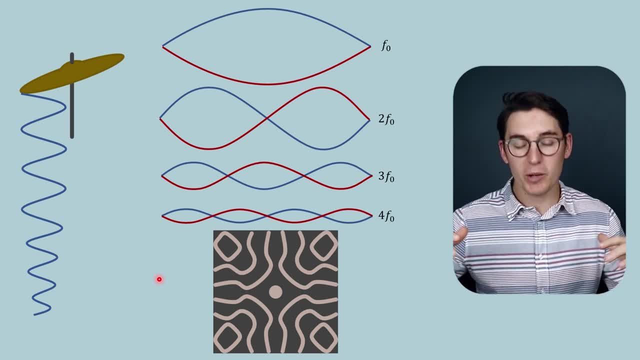 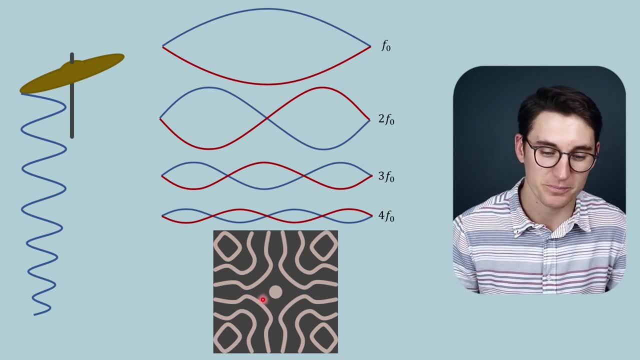 we were to change the note change, that fundamental frequency, we would see the pattern on top of that speaker change And I'd encourage you to go and look at those YouTube videos. I'll link one below in the description. Now, when we are, 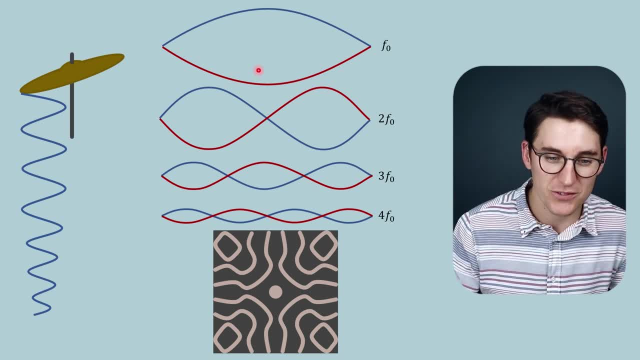 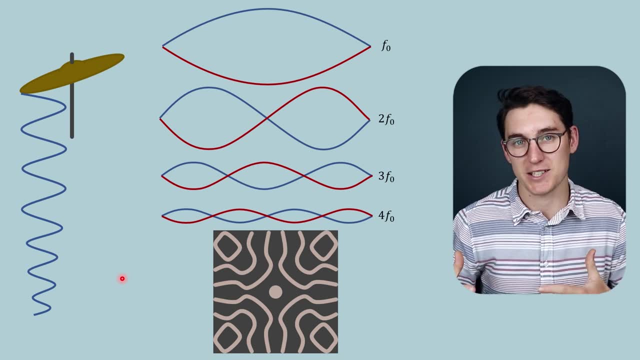 creating ultrasound waves. it's quite difficult to imagine these fundamental and harmonic frequencies because not only are we creating a 2D pulse, we are also propagating that through time and space. We've got a three-dimensional wave being formed here And it's very difficult to visualize the harmonic 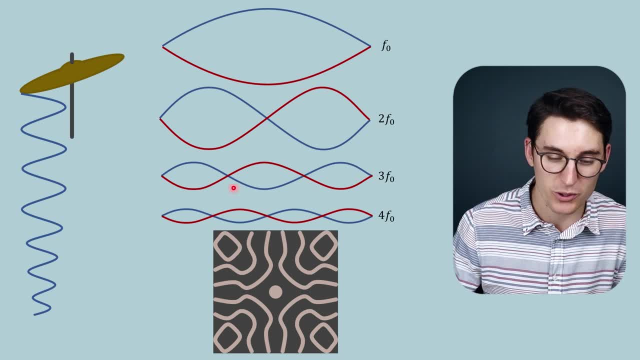 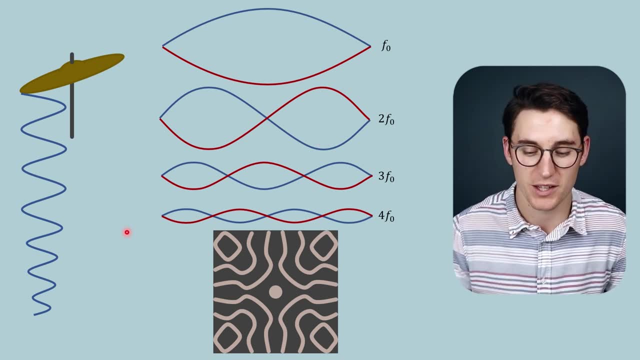 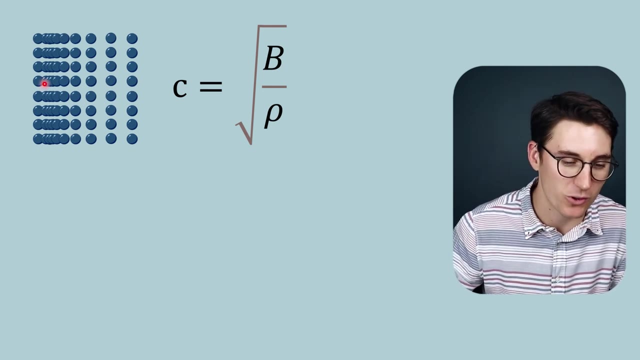 frequencies returning in a three-dimensional wave And it's helpful to return back to this one-dimensional wave as a good conceptual understanding of how fundamental and harmonic frequencies work. Now we've been looking at an ultrasound wave as a longitudinal wave passing through a medium. It requires a medium, it requires units in that medium. 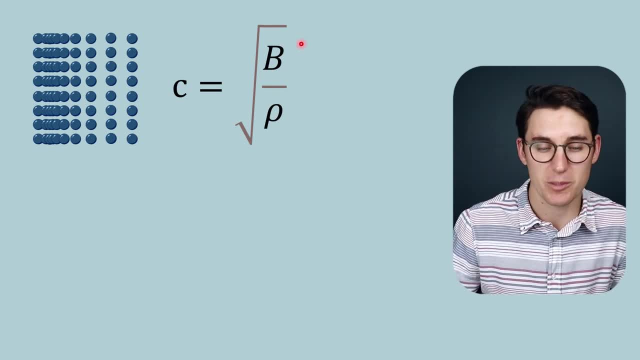 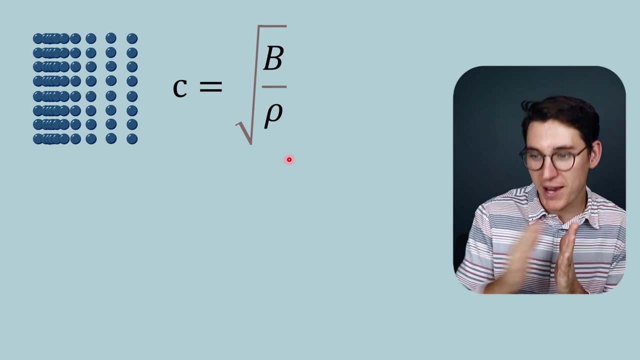 to propagate, And we've seen that the speed of that wave is dependent on the bulk modulus and the density of the tissue through which the ultrasound wave is traveling. The speed is dependent on the tissue through which it's traveling And we've represented this longitudinal wave as a sine wave. 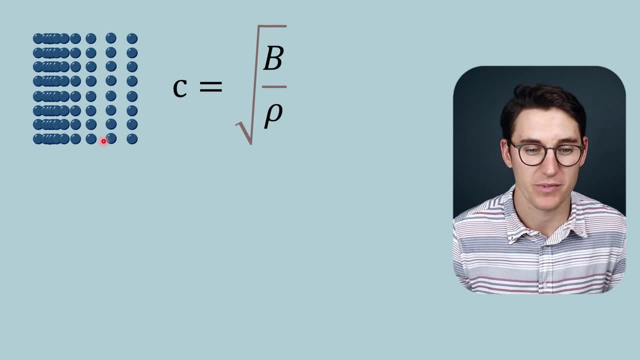 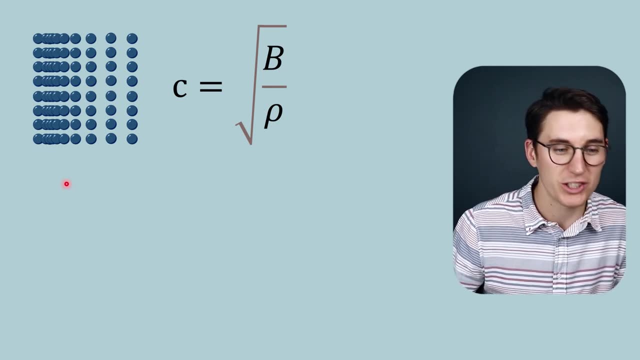 Regions of compression and regions of rarefaction. Now, when we look at these regions of compression versus the regions of rarefaction, we'll see that in the compressed region the molecules or units in that medium are closer together. Now, when those units get closer together, the bulk modulus of that piece of tissue 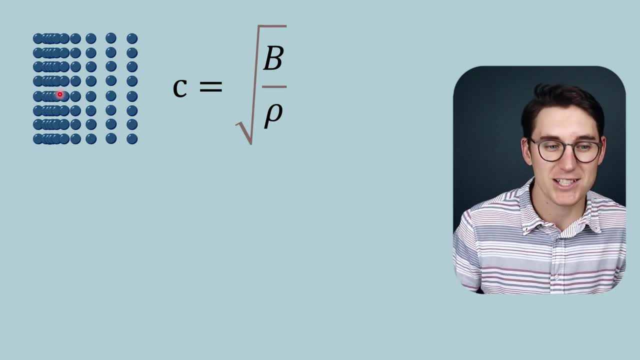 changes- The compressibility gets less or the stiffness of the tissue gets more. It's much more difficult to further compress these units within the medium. When we look at the region of rarefaction, our bulk modulus actually decreases And it's this slight change in bulk modulus that means the 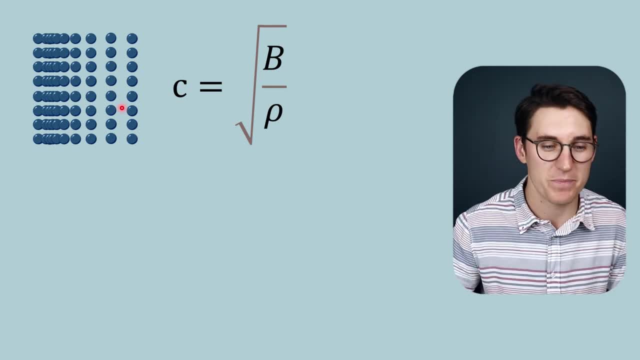 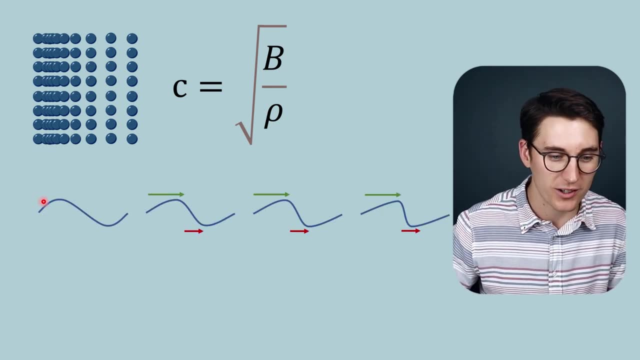 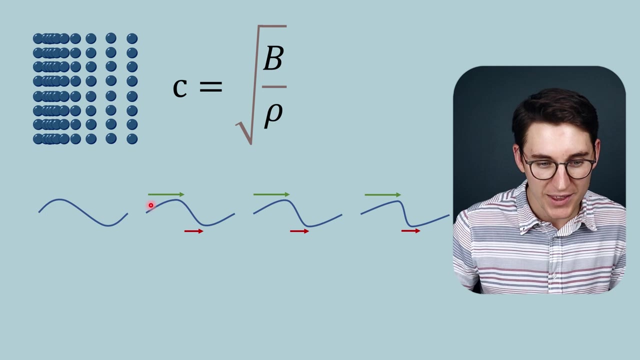 regions of compression actually move slightly faster than the regions of rarefaction, as an ultrasound wave propagates through tissues. So initially we draw our ultrasound wave as the sinusoidal wave And because of the changing bulk modulus in the regions of compression, the compression region on our sinusoidal wave will be moving faster, relatively speaking. 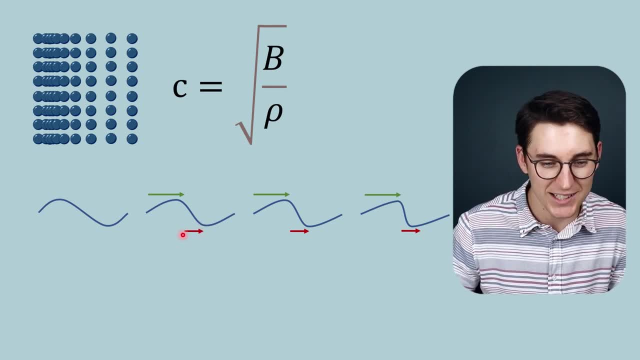 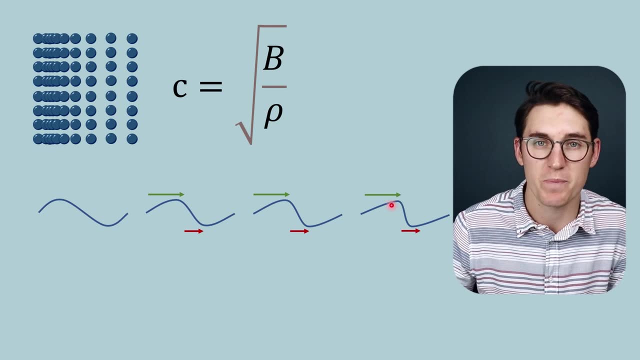 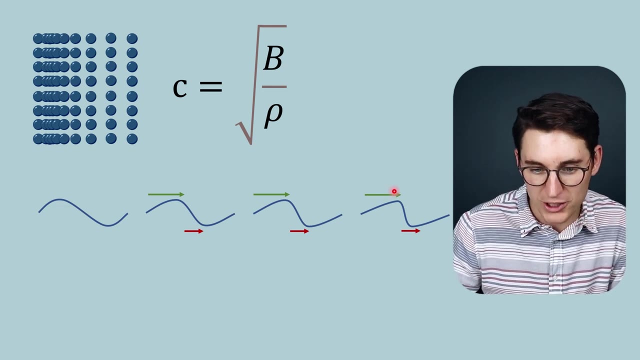 to the rarefaction region here, And it's this slight difference in speed, as that ultrasound wave is propagating through tissue. that means we get this non-linear distortion of the ultrasound wave. This is what's called non-linear behavior in an ultrasound wave. The regions of compression. 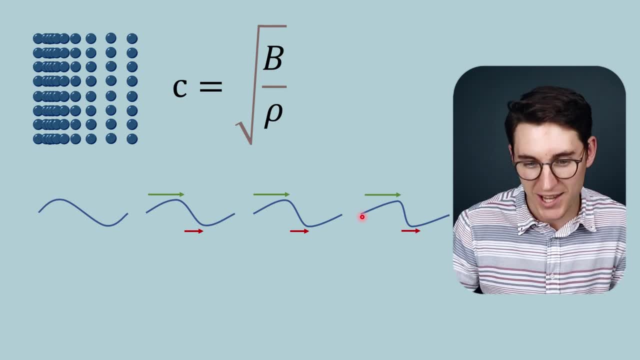 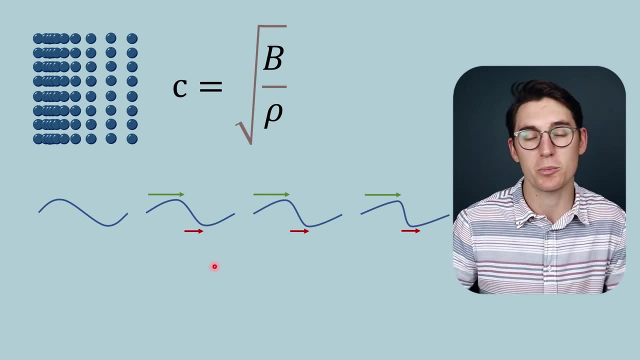 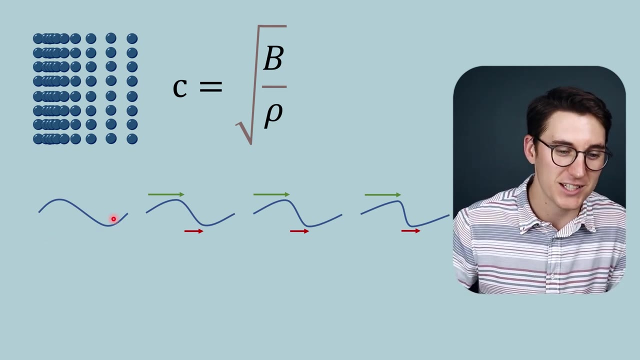 are moving slightly faster than the regions of rarefaction and we get this distortion, this non-linear behavior of the ultrasound wave. Now, this is the basic principle for why we get harmonic frequencies returning back to the ultrasound machine. If the wave remained in its sinusoidal waveform, we would only get the fundamental frequency returning from tissue. 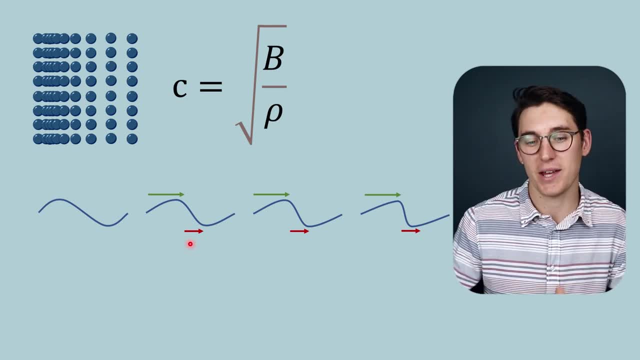 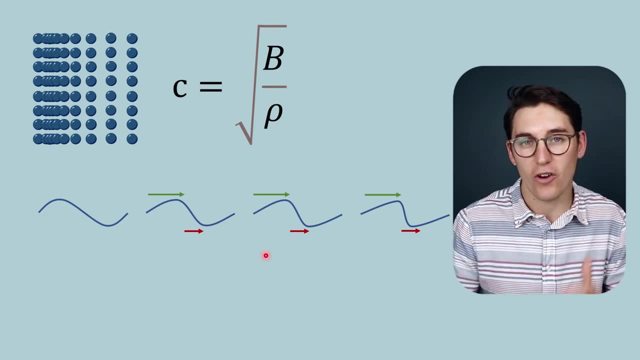 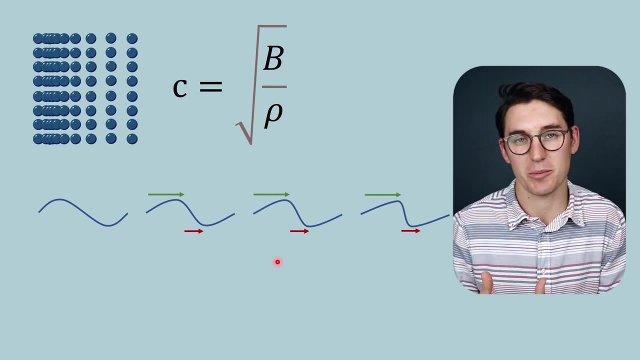 boundaries. As the wave exhibits this non-linear behavior, we start to get harmonic frequencies returning to the ultrasound machine, And this only happens in regions of high intensity within our ultrasound beam. Now, this is the first reason for why we would get harmonic frequencies returning. 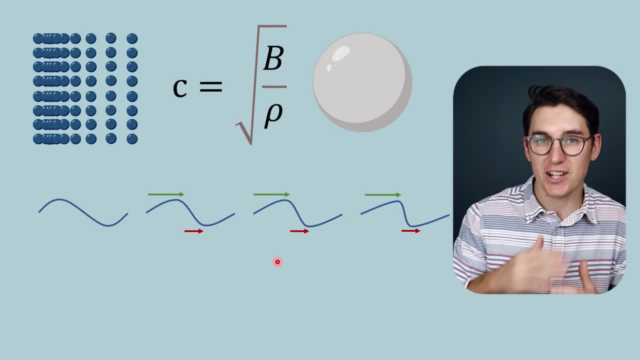 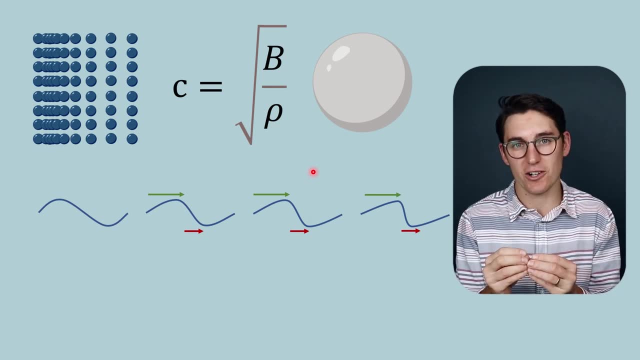 back to the ultrasound transducer. The second reason is if an ultrasound wave comes into contact with what is known as a micro-bubble, When this bubble of air is smaller than the wavelength itself, it will expand and contract based on these regions of compression and rarefaction. And that expansion and contraction. 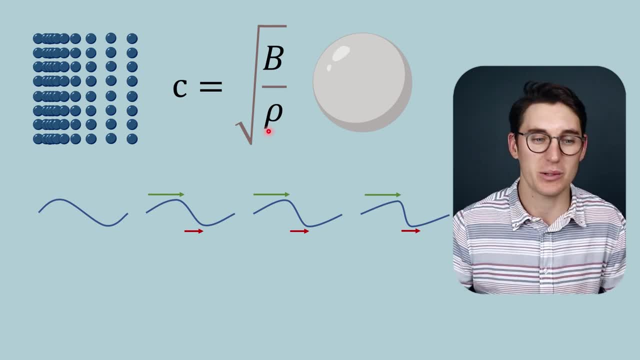 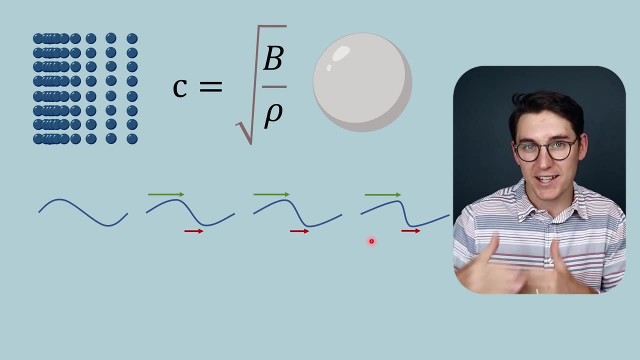 will cause this bubble to resonate at a harmonic frequency to the incident ultrasound wave, emitting harmonic frequency waves back to our ultrasound transducer. Now we're going to be focusing on tissue harmonics here. it's actually the tissue's response to this ultrasound wave that is causing those harmonic. 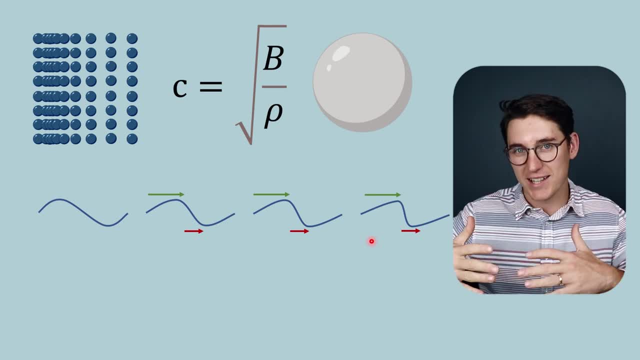 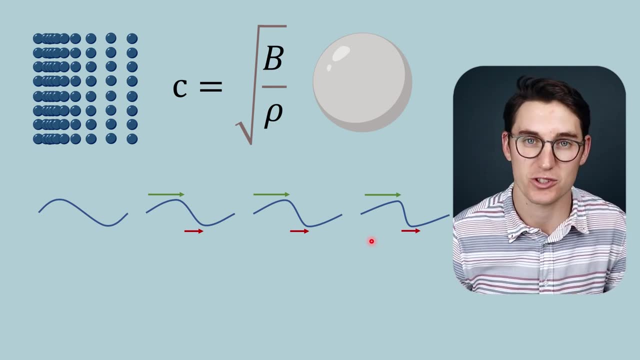 frequencies. to return to the ultrasound pulse, You can think of that tissue as resonating at a harmonic frequency and creating a separate ultrasound pulse that is heading back towards our transducer Now, because this non-linear behavior of the ultrasound wave happens as the wave is. 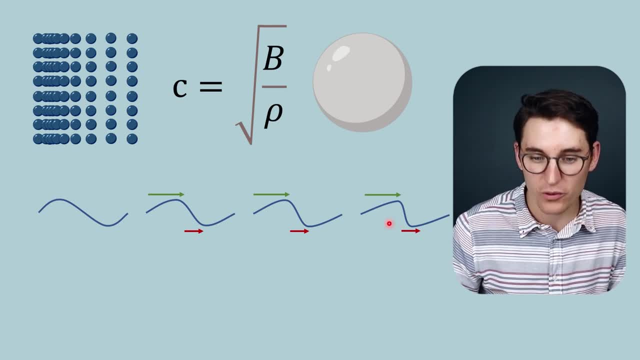 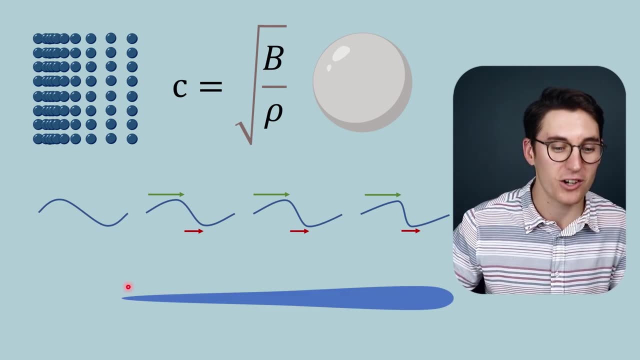 traveling through tissue, we get more and more production of harmonic frequencies as that wave travels deeper into tissues. So the quantity of harmonic frequencies that we get is going to be the frequency that is going to go in después de ahora. This energy of demonicimporte that are returning to our ultrasound probe increases with depth within the tissue. 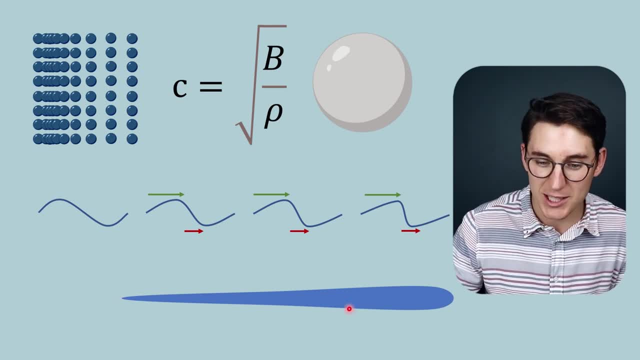 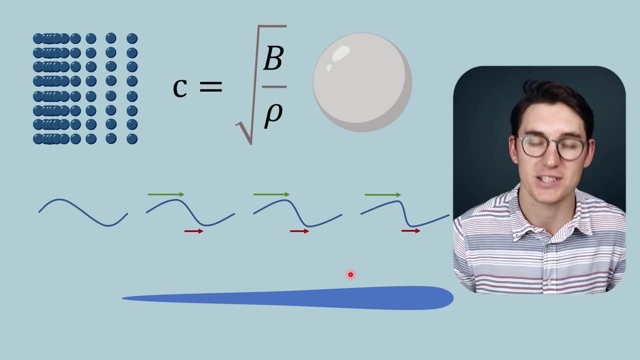 we start off with very few harmonic frequencies returning to the transducer probe and as we get deeper and deeper into the tissues we get more and more harmonics, first, second, third, fourth order of harmonics being formed deeper into the tissue. Now we can superimpose this over our ultrasound beam. here 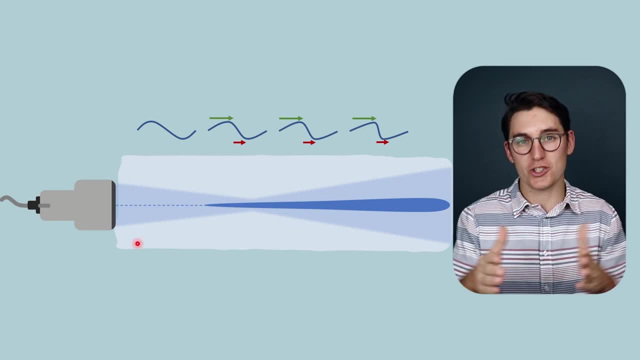 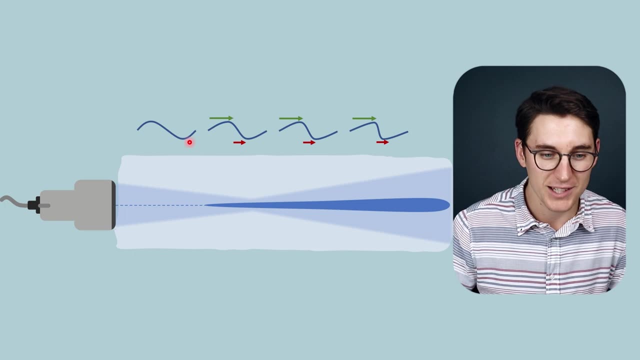 we can see that our ultrasound beam is traveling through tissues, with our near field and our far field with our, from our ultrasound end itself, based on細 mi kimba signal focal zone here, as we've seen before when we looked at the ultrasound beam. Now, because of this, 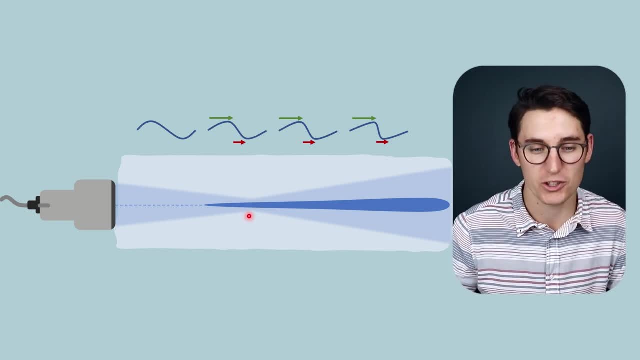 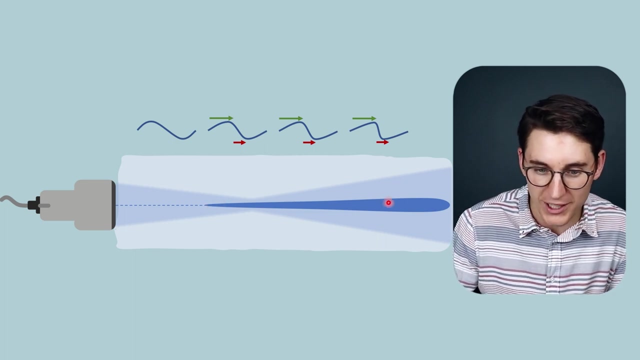 non-linear behavior of that ultrasound beam propagating through tissue, we start to get harmonic formation deeper into the tissues. Now I mentioned- and this is really important- harmonic frequencies only happen at intense parts of the ultrasound beam and that's why we can see we only get harmonic formation here, in the center of our beam, the most intense region of our beam. We are. 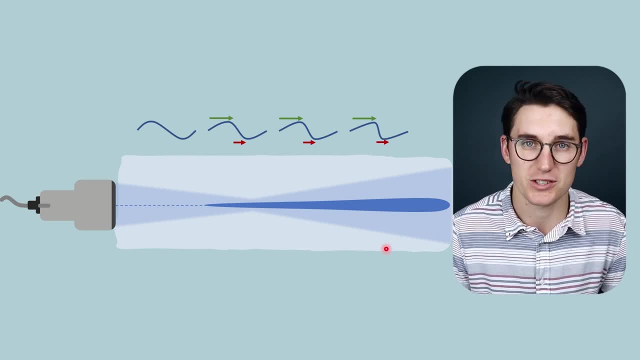 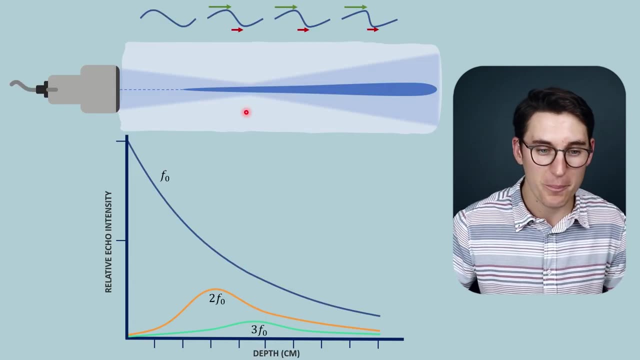 not getting harmonic frequencies on the lateral portions of the ultrasound beam. here Now we can plot the various different harmonic frequencies that are returning to our transducer on a graph based on how deep we are within the tissues. Initially we have our fundamental frequency, the pulse echo frequency that we've been looking at throughout this ultrasound course. 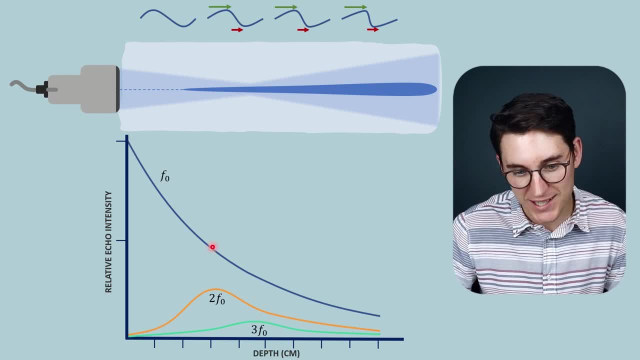 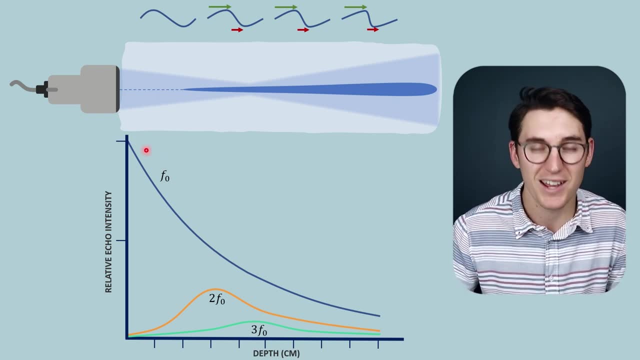 and, as we've seen before, that pulse echo gets attenuated as it travels into tissue here and that attenuation is dependent on the frequency of that ultrasound beam. Now we can plot the various different harmonic frequencies that are returning to the ultrasound wave. The higher the frequency, the more it gets attenuated. Now, as you can see here, 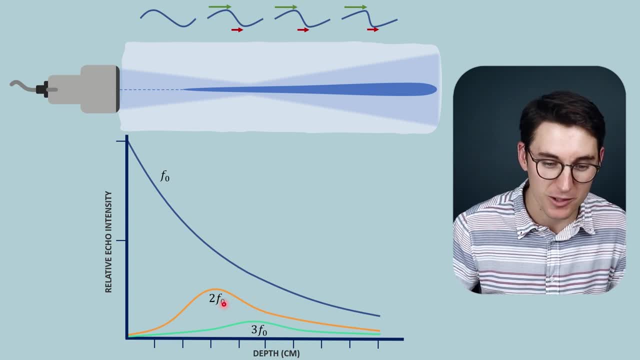 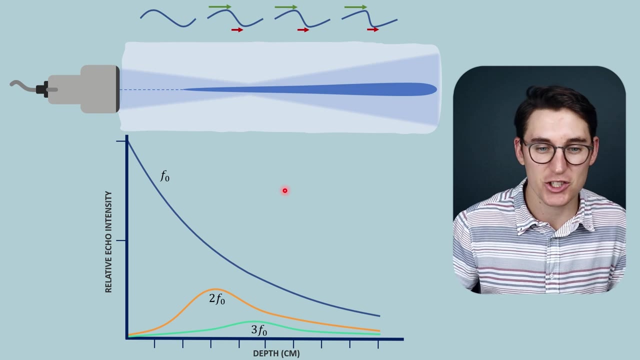 we get first order harmonic frequencies or two times our fundamental frequencies, forming just before the focal zone of our ultrasound beam here and we can see that as we travel further into the tissue we start getting a peak of this first order harmonic. As we travel deeper into the tissue we 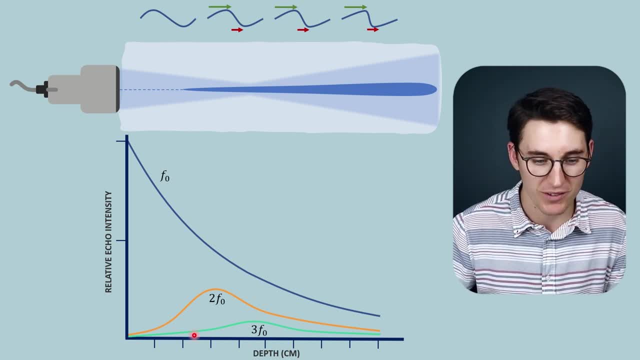 get more and more non-linear behavior of this ultrasound wave and we start to see second order or three times more non-linear behavior of this ultrasound wave. Now we can see that as we travel further. it's only the minimum frequency of the second order, harmonic, which is actually three times the fundamental frequency. 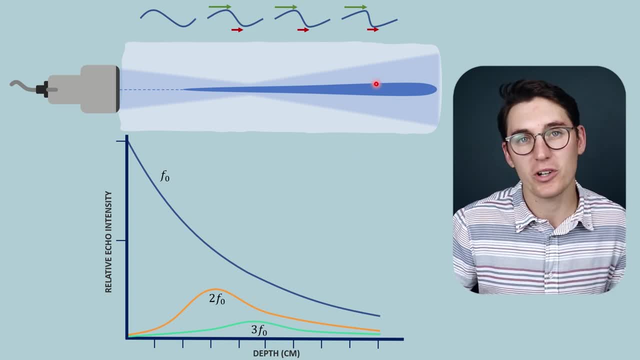 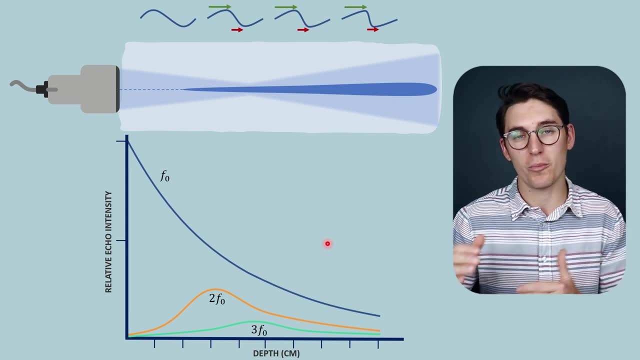 returning back to our ultrasound probe Now, although we are returning more harmonic frequencies, the deeper we head into the tissues. those harmonic frequencies- the second and third order harmonics- are very high frequency ultrasound waves and they won't be able to make it all the way back to our ultrasound. 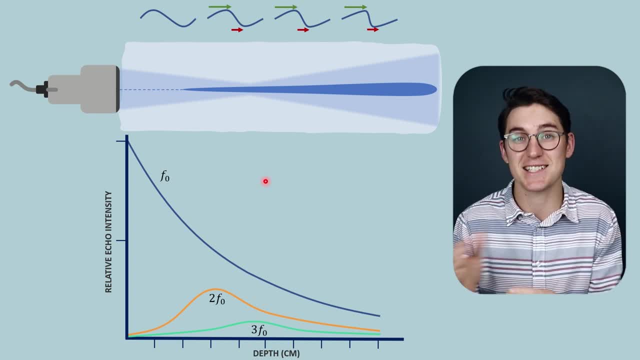 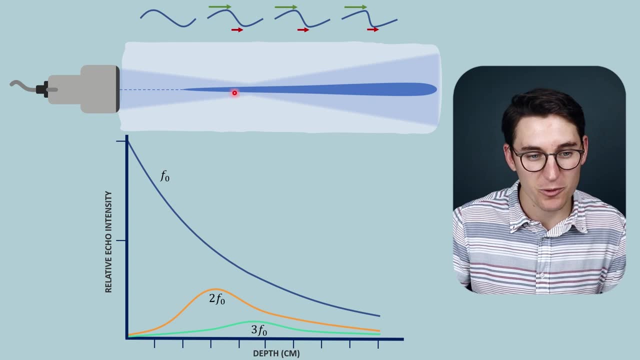 transducer because high frequency ultrasound waves get attenuated quickly. So although we're creating a lot of higher order harmonic frequencies, those aren't very useful to us because they don't make it back to us. So I'll leave the that up for discussion for a while and we'll come back to a bit more detail in the following slides. 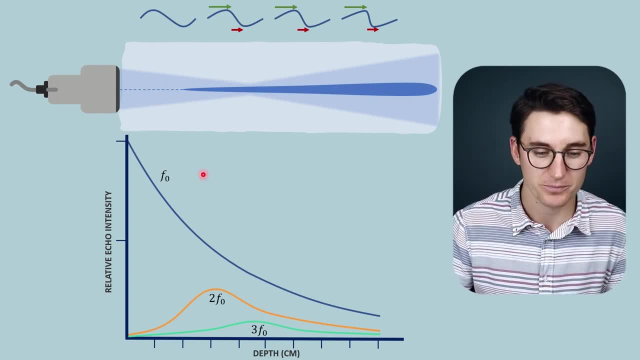 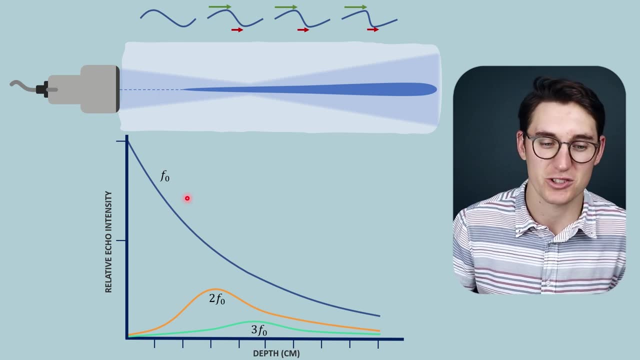 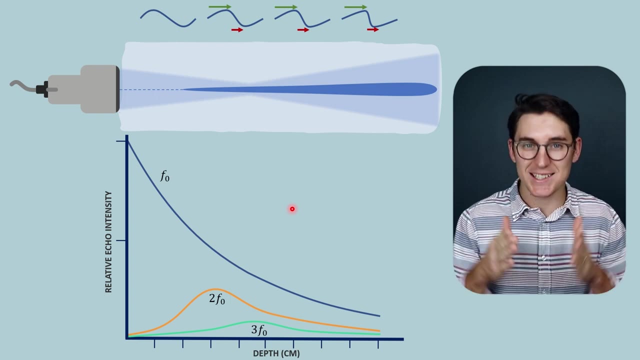 to the ultrasound transducer. They're attenuated before they can travel back, And we generally focus on this first-order harmonic- two times the fundamental frequency of our ultrasound transducer. Now, why do we focus on harmonic frequencies? Well, harmonic frequencies- one only- occur at 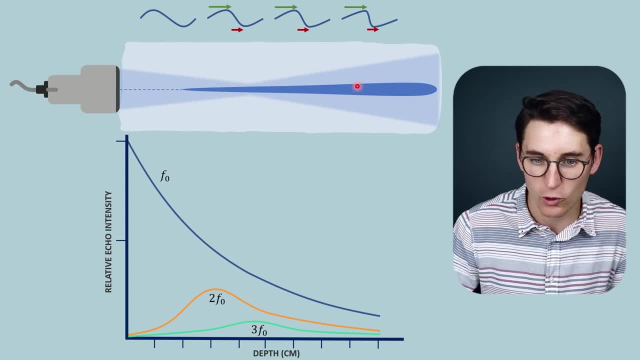 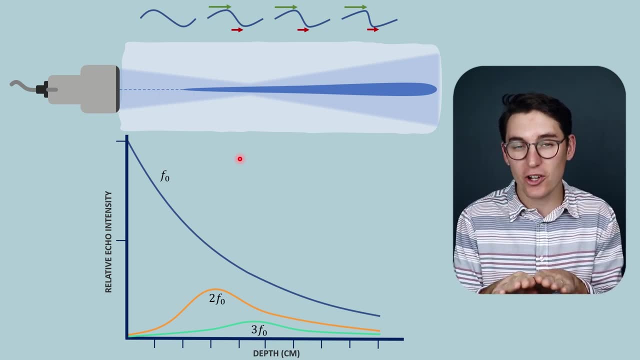 the intense parts of the beam. We've got a very narrow beam being formed here. We get great lateral resolution here And two harmonic frequencies: tissue harmonic frequencies only occur at tissue boundaries. They're created by the tissues. It's true signal heading back to. 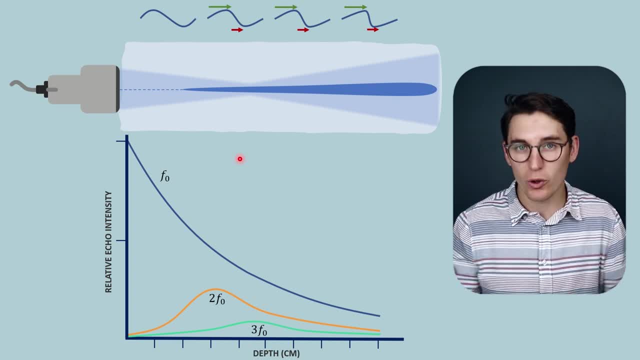 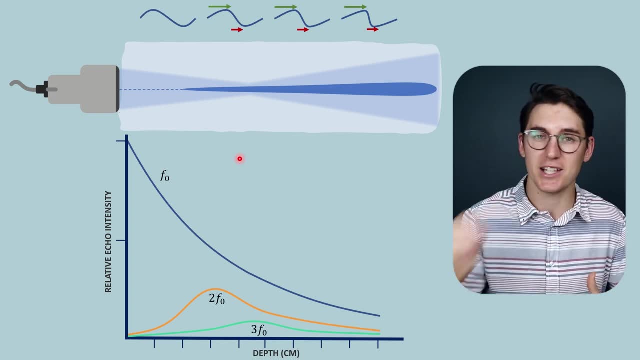 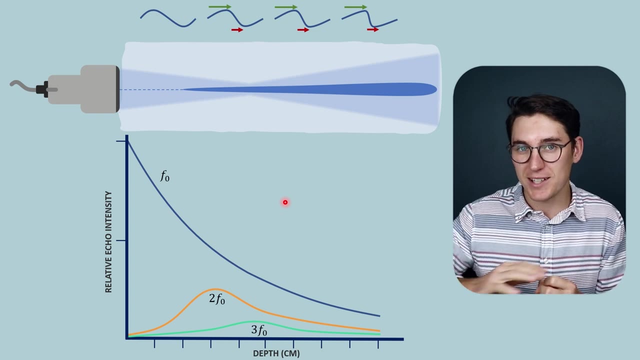 our ultrasound transducer. The scatter that happens or the noise that happens in a normal beam mode, ultrasound image aren't at harmonic frequencies And if we can select specifically for those harmonic frequencies that are returning back to our ultrasound transducer, we get true signal heading back. We can eliminate some of that scatter, eliminate some of that. 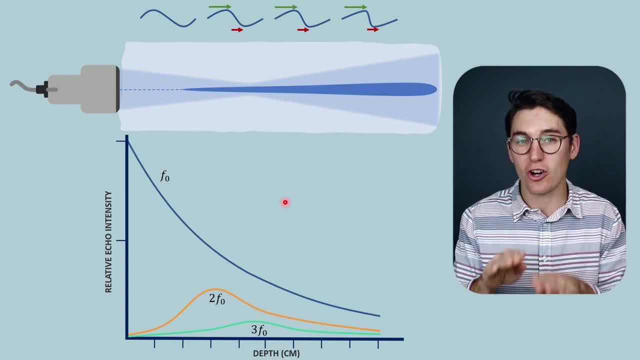 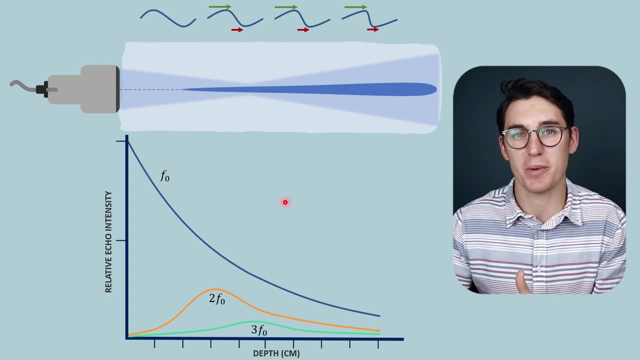 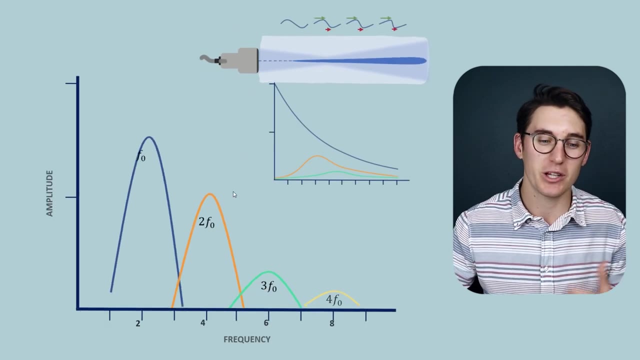 background noise, get better spatial resolution and ultimately, better contrast within our ultrasound image. What we see on that beam mode image more accurately represents the true tissue boundaries within the tissues. Now, if we take a specific point along this ultrasound beam, we can see the types of frequencies that are returning back towards our 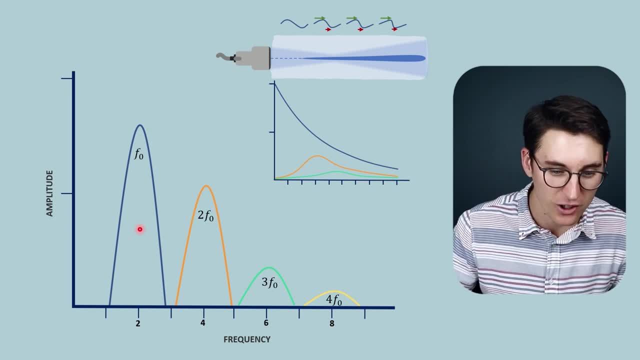 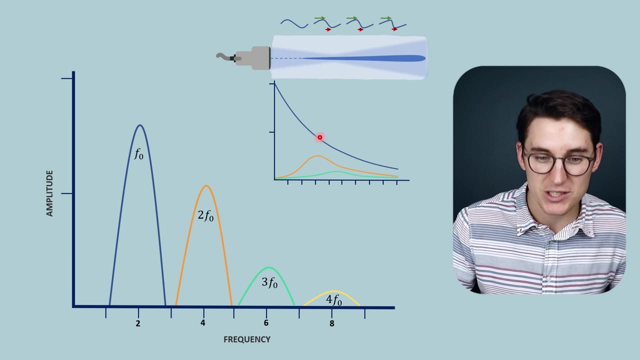 ultrasound transducer. Say this transducer was a two megahertz transducer, we would get a first order frequency of four megahertz, then a second order of six and a third order of eight megahertz. And we can see that if we take a specific point along this beam, the majority of them are still. 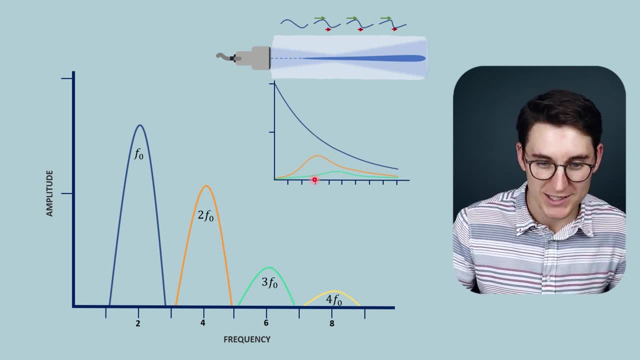 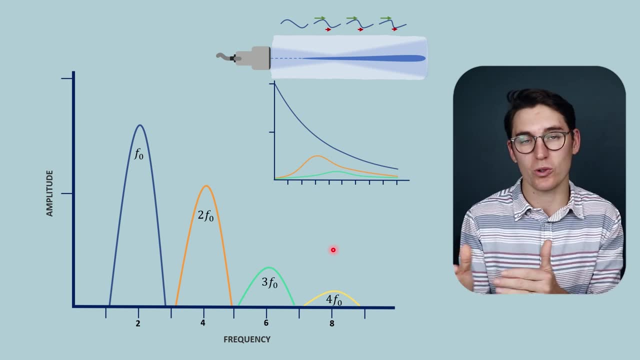 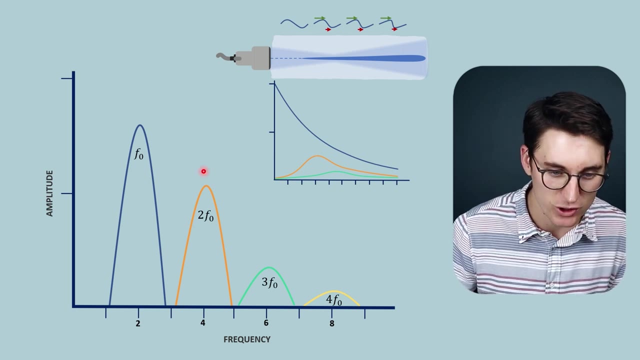 the fundamental frequency. but we're getting first order and second order harmonic frequencies returning to the ultrasound machine And we want to now isolate these specific first order harmonic frequencies returning. They best represent the tissue boundaries. Now there are three main ways that we can isolate this first order harmonic frequency. Now, this only works if we know what. 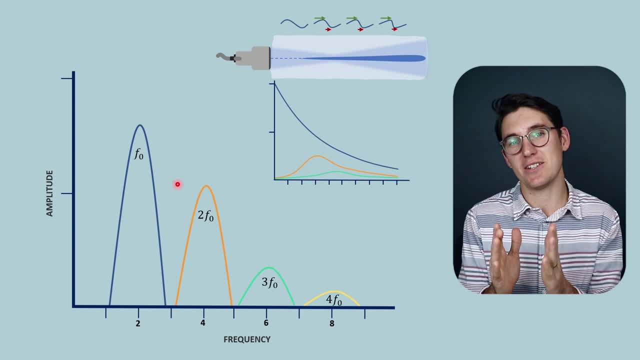 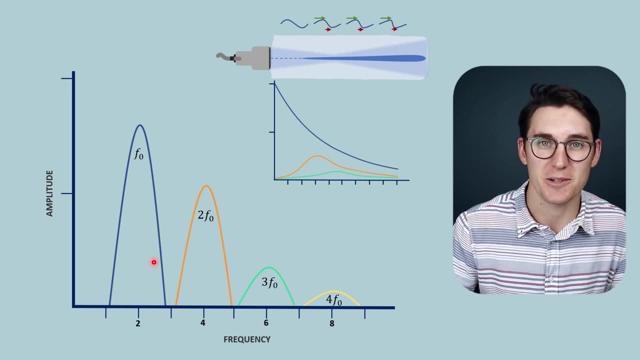 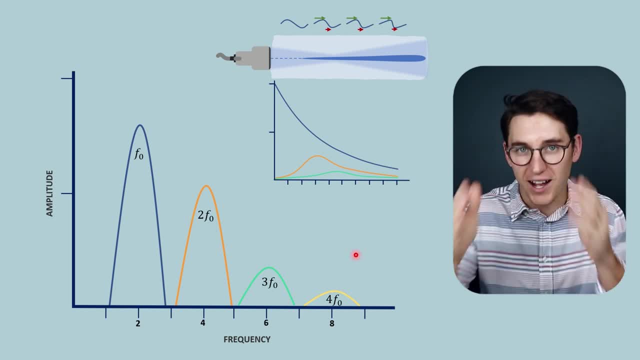 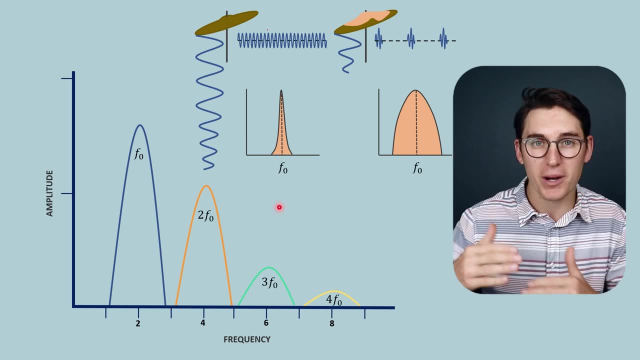 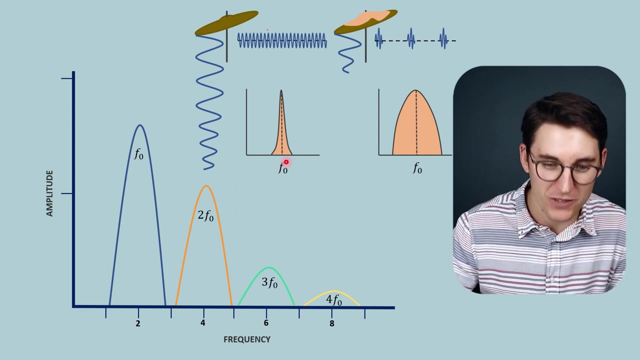 integer values of this fundamental frequency. Now, how do we create a high quality wave? We've seen this before. We can increase our spatial pulse length, We can allow that piezoelectric material to resonate at its resonance frequency and that will give us a narrow bandwidth, a very specific 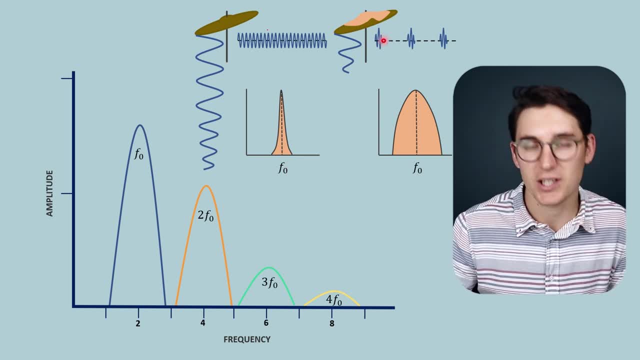 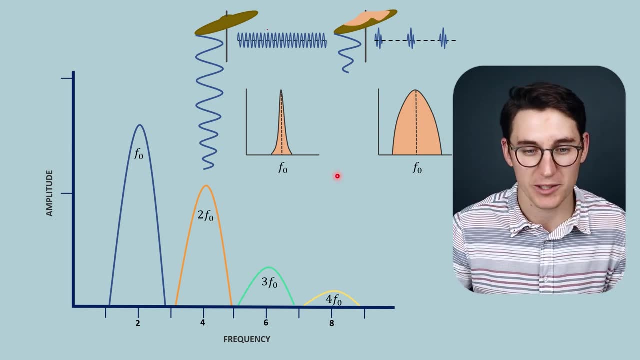 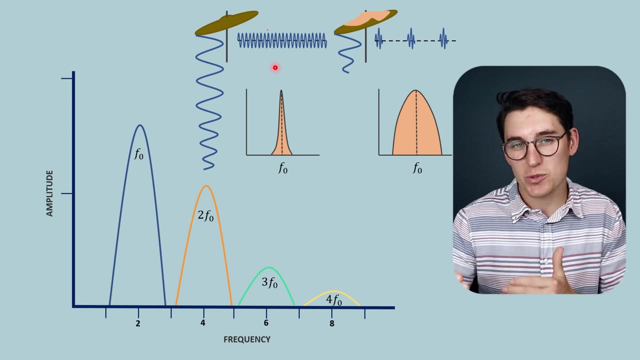 frequency heading into it. The shorter and shorter our spatial pulse length, the wider the bandwidth and the less pure the harmonic frequencies are that are returning towards our ultrasound machine. Now the problem with having a high quality factor wave, a undampened wave that has a long spatial pulse length, is we get a reduction in axial 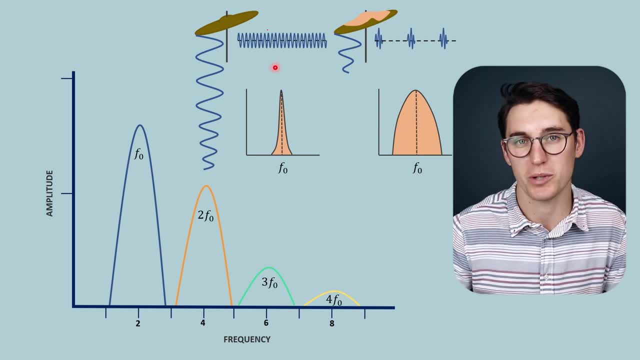 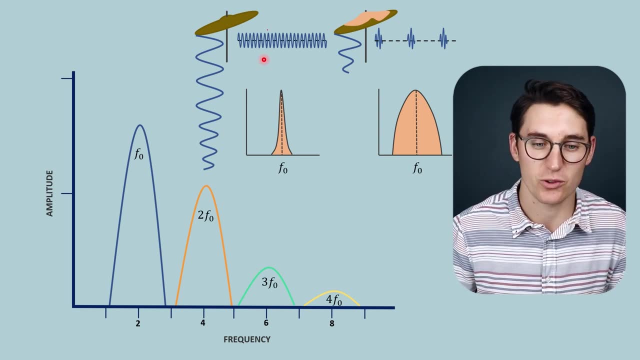 resolution. We've seen that axial resolution is dependent on the spatial pulse length, So it's a little bit of a trade-off. How pure can we make the frequencies heading into the tissue without losing too much axial resolution? And we'll see how we can do that. 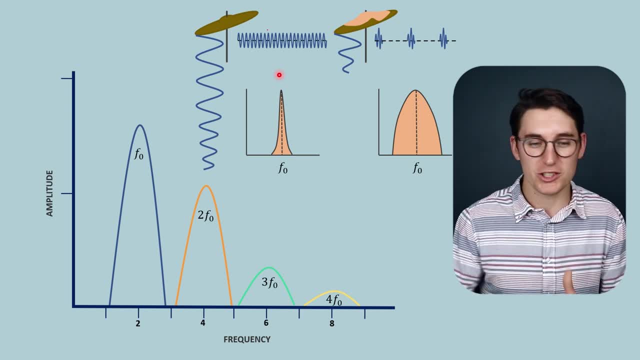 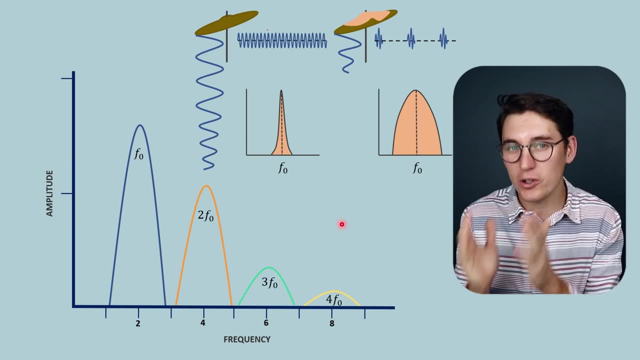 We're going to get back some of that axial resolution now. Now what we want to do is isolate this specific first order harmonic frequency that's heading back towards our ultrasound transducer and only use those returning echoes to create our beam mode image. That image is going to have much better contrast and spatial. 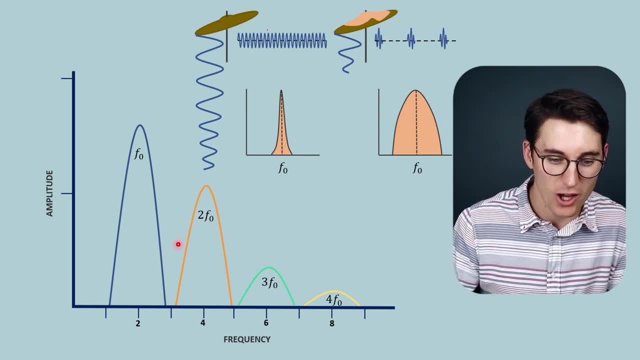 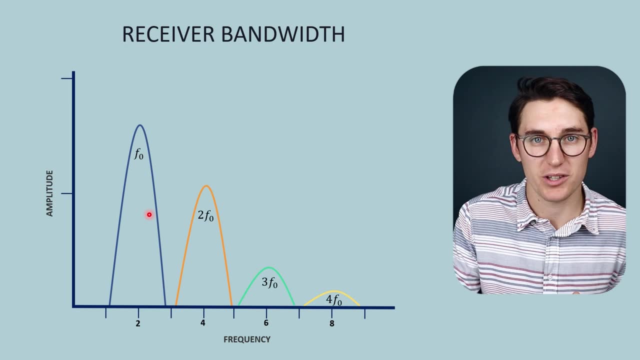 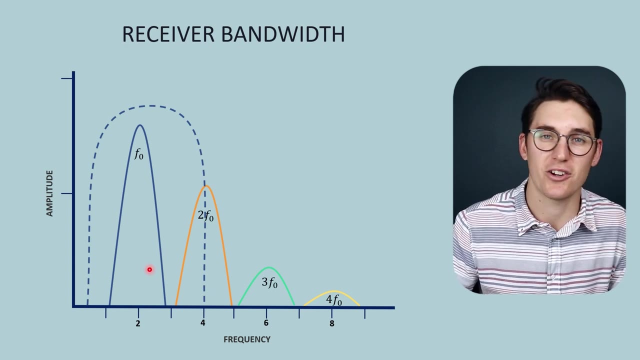 resolution. Now there are three main ways that I want to talk about today for isolating this specific harmonic frequency. Now the first way we can do it is by changing the receiver bandwidth. When we have a 2 MHz ultrasound transducer, we will generally have a receiver bandwidth that flanks the 2 MHz here And we will receive any echoes. 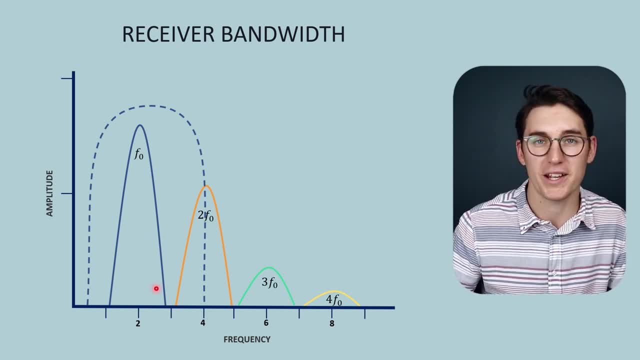 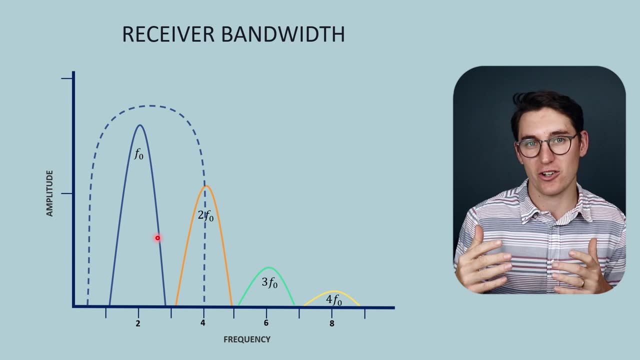 returning from the tissues that lie between this 1 and 4 MHz. here, for example, We've got a fairly wide receiver bandwidth so we can get all those scattered echoes, we can get those tissue boundary echoes and we'll get some of the 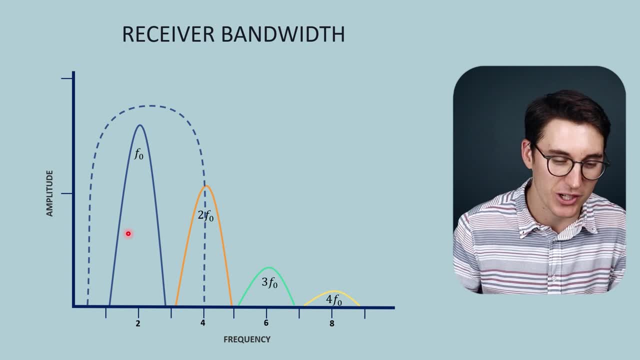 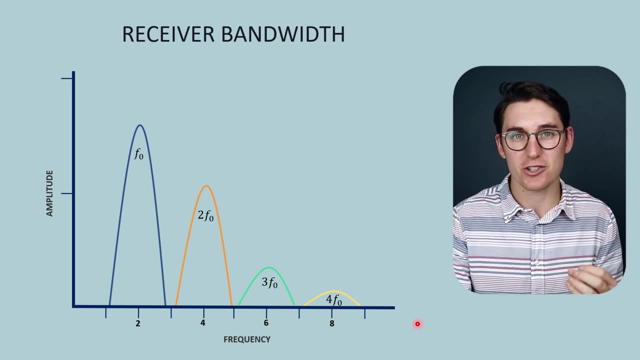 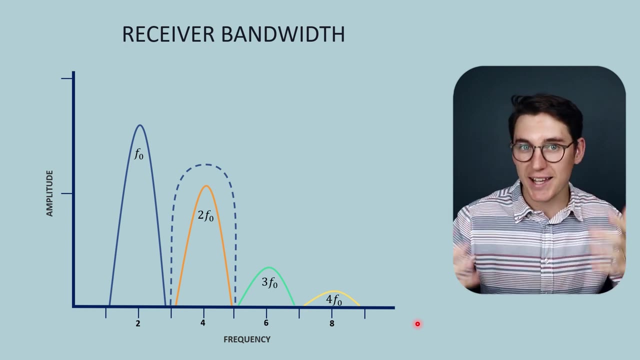 noise coming back from our tissues And this is how we traditionally create our pulse, echo ultrasonography image. Now what we can do is actually change that receiver bandwidth. We can say to the ultrasound machine: only listen for echoes that are returning at 4 MHz in frequency. Now what that does? we're still getting all those. 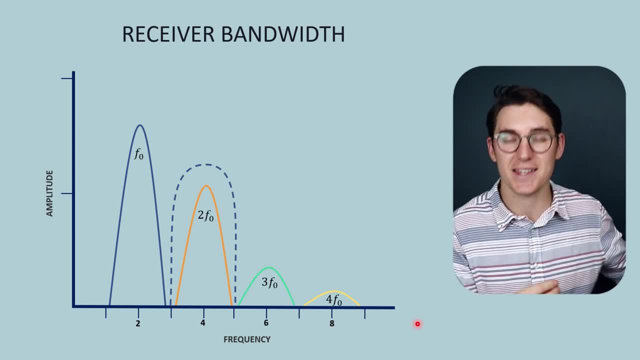 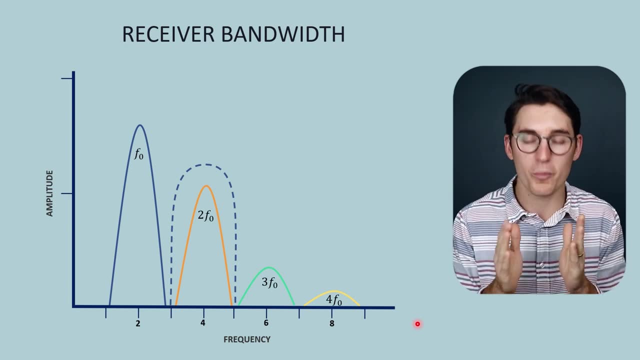 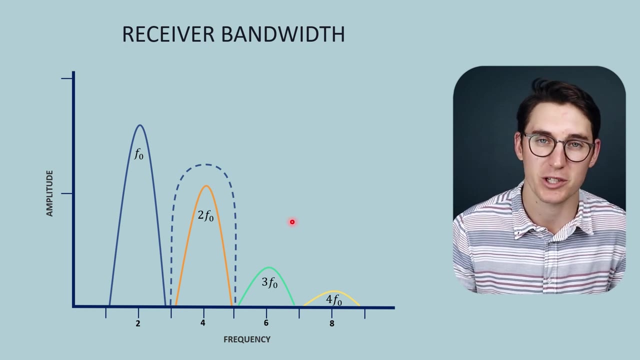 other echoes back, but electronically, when we're sending signals via the amplifier towards the machine for processing, for displaying that beam mode image. we only want to process and display 4 MHz, We only want to display the harmonic frequency, the first order harmonic frequency here, two times the fundamental frequency That allows us to only 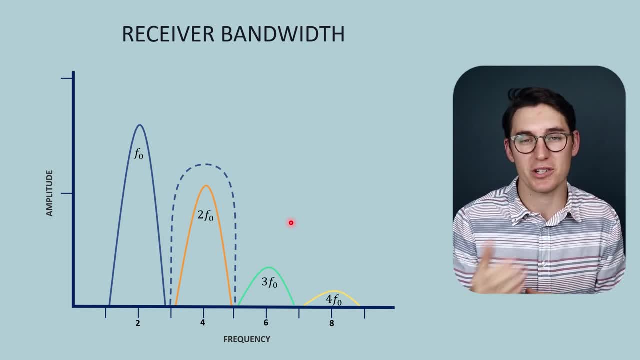 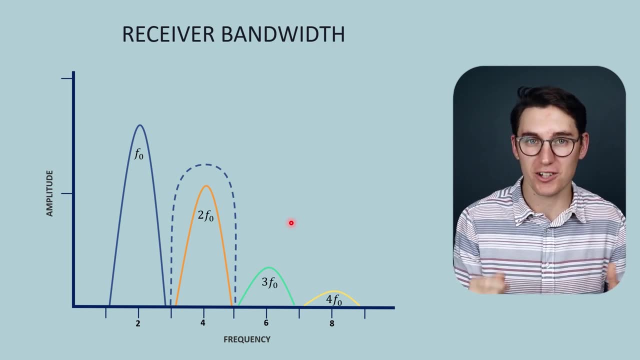 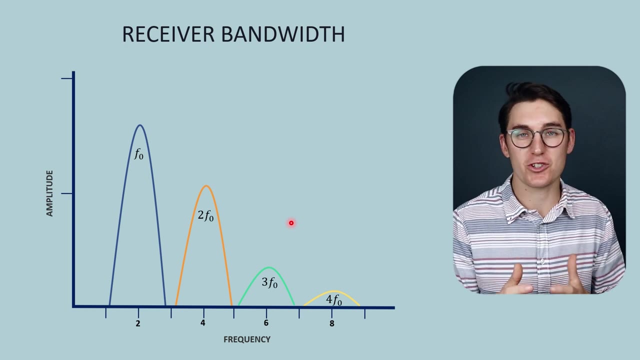 display harmonic frequencies coming back, True tissue bandwidth, True tissue boundary frequencies. Those harmonic frequencies have been created within the tissue. Now, when you set harmonic mode on the ultrasound machine itself, it will automatically do this. it will narrow down the receiver bandwidth. Now this requires the ultrasound machine to pull out only those returning echoes. that have our first order. 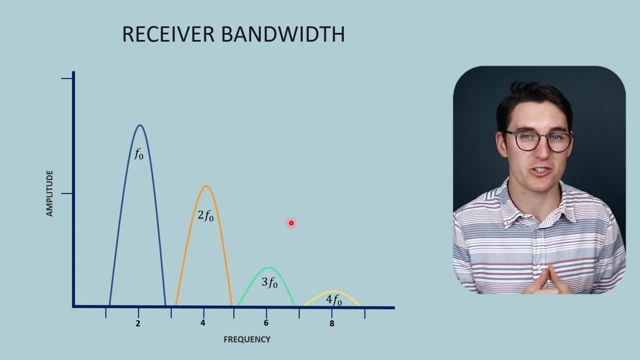 harmonic in them. It requires that fast Fourier transform that we've mentioned before. Now there are other ways that the machine doesn't have to manipulate the data returning and it will only get harmonic frequencies from. the is coming back predominantly to the ultrasound machine, and the first way we can do this is what: 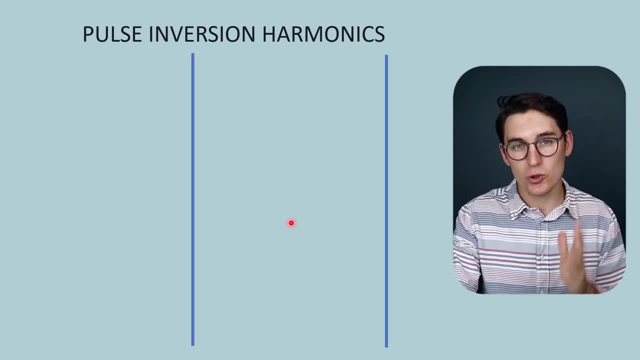 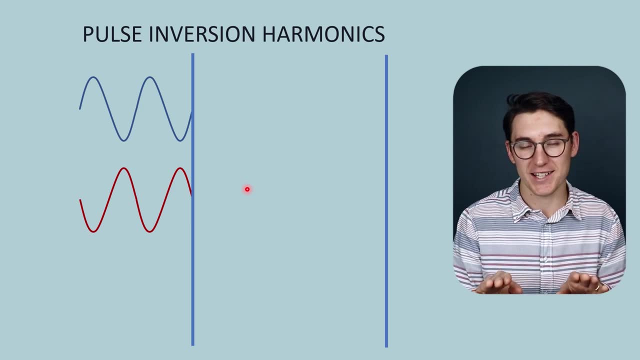 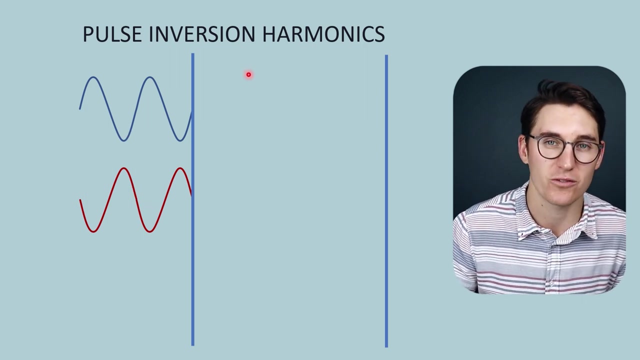 is known as pulse inversion harmonics. we can send two separate pulses down an individual a-line towards a tissue boundary. here now the pulses are out of phase. they're 180 degrees out of phase. the second pulse is an inversion of the first pulse. that's why it's called pulse inversion. 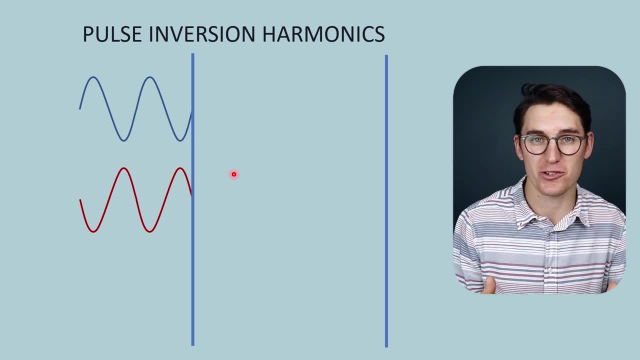 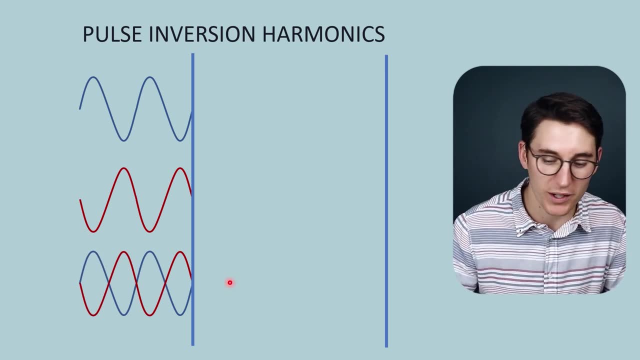 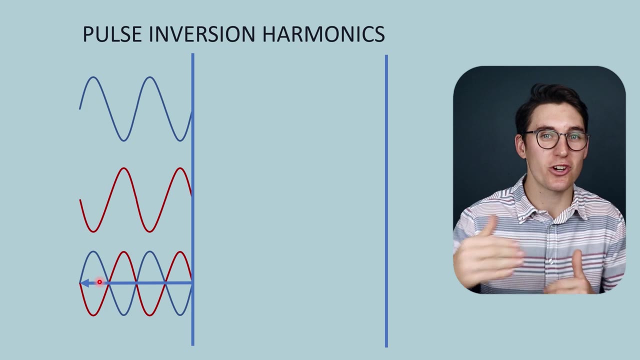 harmonics. those pulses head towards a tissue boundary at the fundamental frequency and they will create echoes at the fundamental frequency that will cancel one another out. there will be destructive interference of those echoes. we won't get fundamental frequencies. returning to the ultrasound machine here now, we've also seen that when these pulses travel through a certain depth, 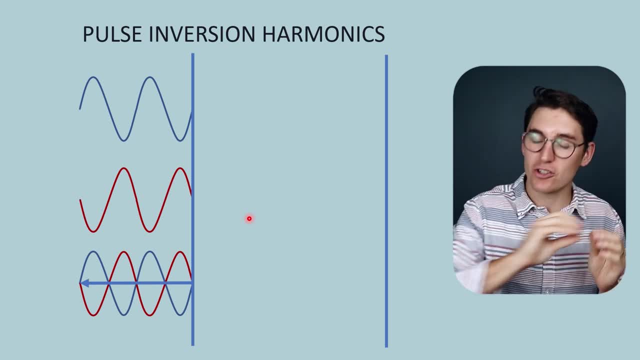 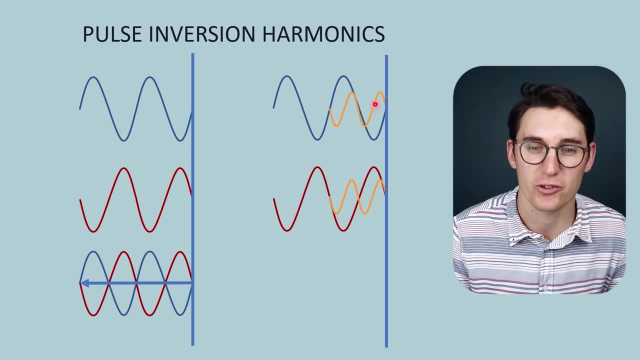 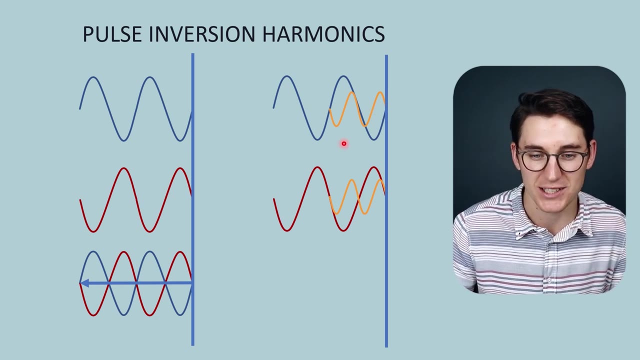 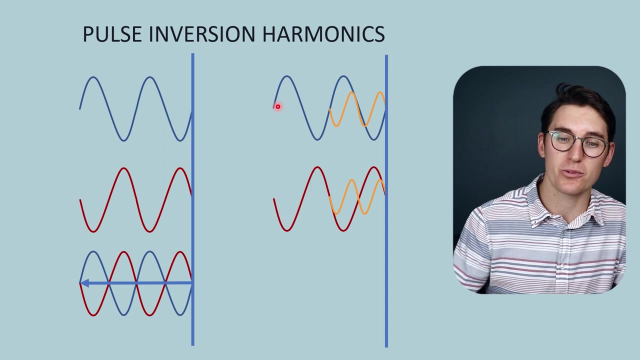 of tissue in an intense part of the wave. because of that non-linear behavior of this ultrasound pulse, they are also going to generate harmonic frequencies at tissue boundaries. the tissue is responding to this fundamental frequency and resonating at a harmonic frequency, an integer multiple of this fundamental frequency. now these echoes coming back at the fundamental frequency, 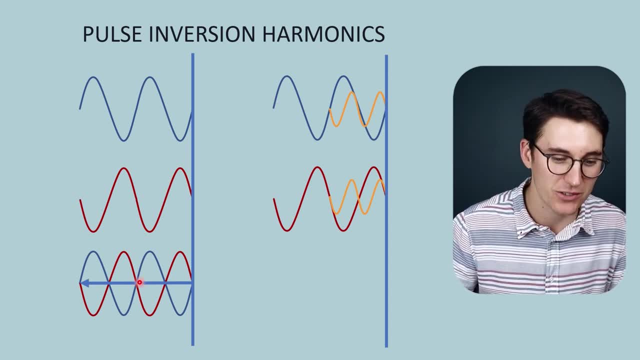 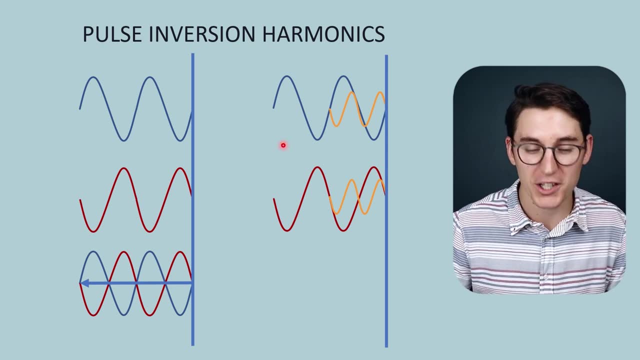 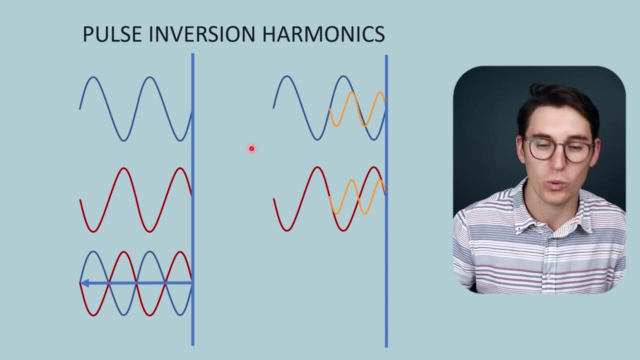 will be inversions of one another and destructively interfere with one another, making no fundamental frequencies head back towards the transducer. now, a property of the harmonic waves that head back from tissue boundaries means that they are going to actually head back in sync, despite the initial waves being inversions of one another. now, if you think back to the first slide, 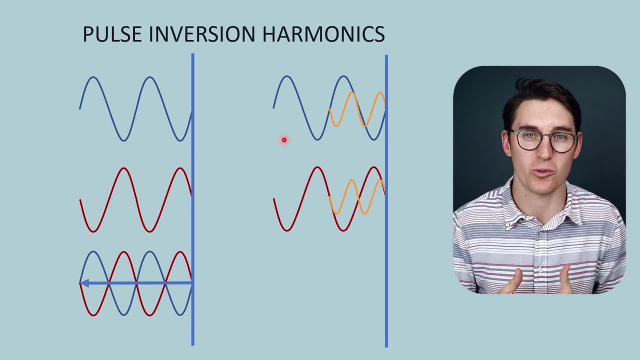 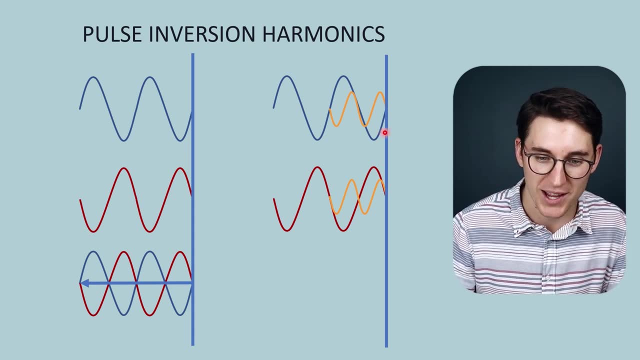 of this talk, when we looked at one, two and three dimensional harmonic ultrasound waves, said it's quite difficult to conceptualize two and three dimensional waves. and this is a property of these waves heading back: they're going to be in phase because the tissue boundaries are essentially 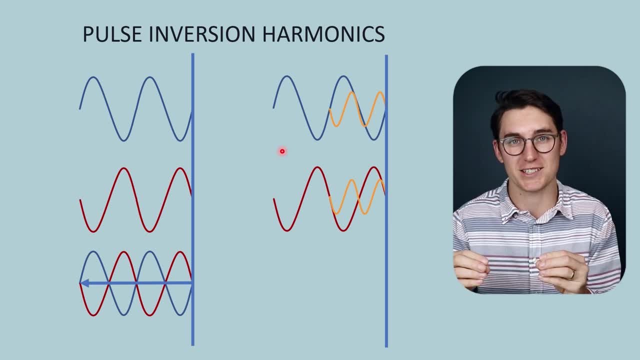 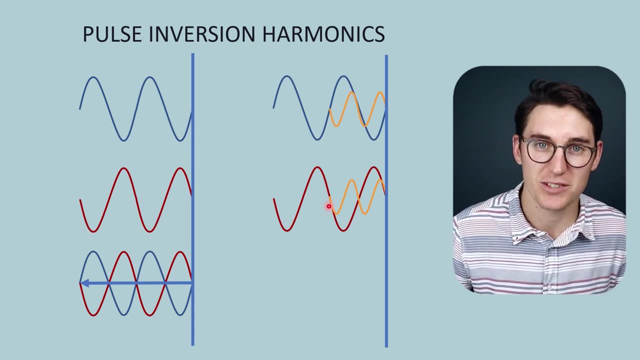 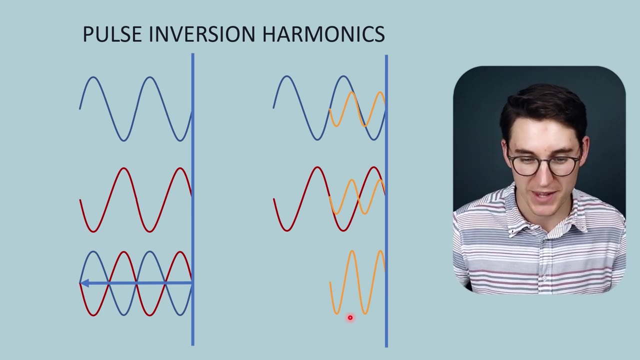 creating these harmonic frequencies. that's why it's called tissue harmonics. the tissue is creating that harmonic frequency heading back to our ultrasound probe, and we're going to constructively interfere with one another and give us a higher intensity harmonic frequency heading back towards the ultrasound transducer and we can use this echo. 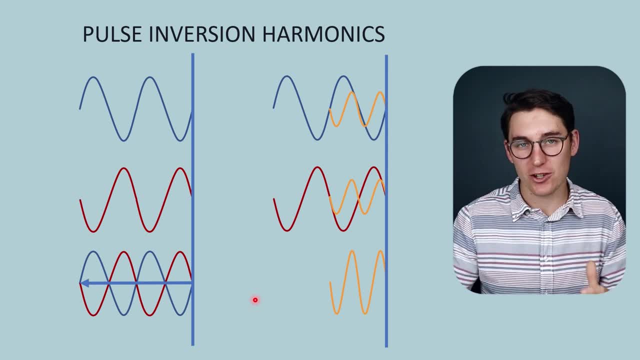 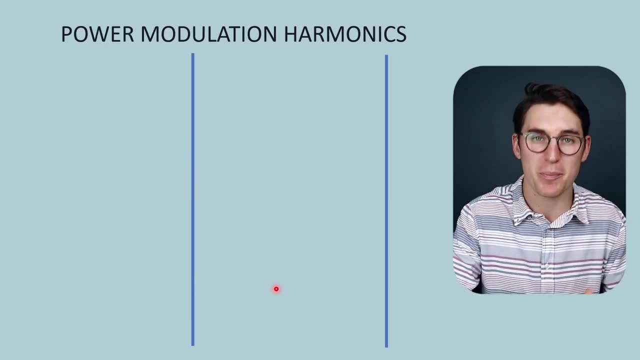 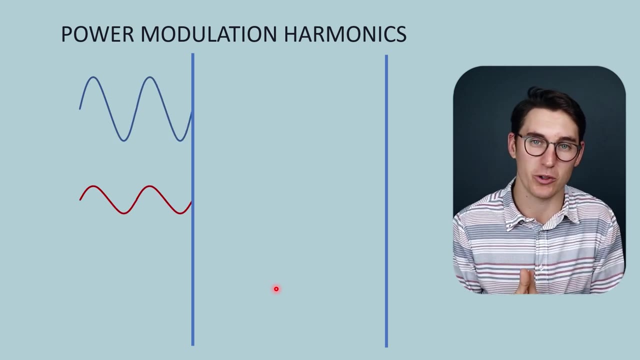 to create our harmonic imaging. now there's one last method that allows the ultrasound transducer to only accept the harmonic frequencies heading back from tissue boundaries, and that's what's known as power modulation harmonics. again, we send two ultrasound pulses down one a-line within our 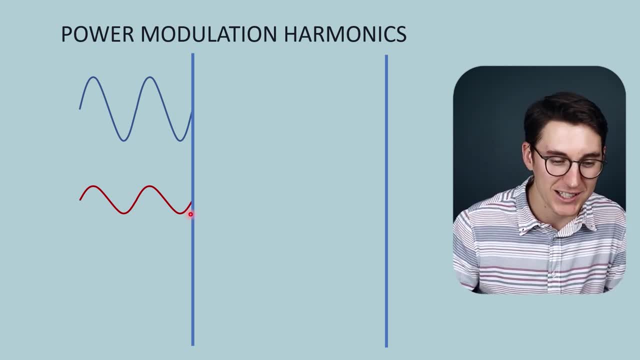 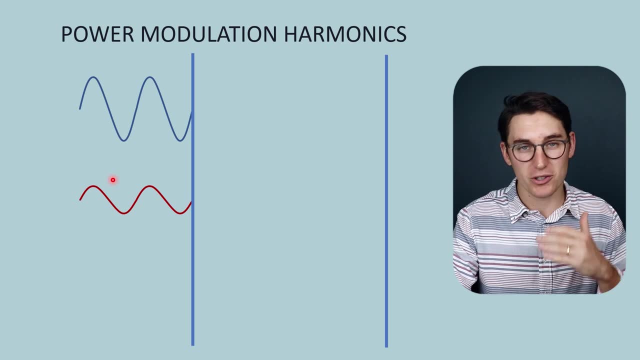 b-mode image. so we do the same with the other two ultrasound pulses. we send down a higher intensity, so we send down an intense ultrasound pulse and a slightly weaker or less intense ultrasound pulse. they still have the same fundamental frequency. now, when these pulses reach a tissue boundary, 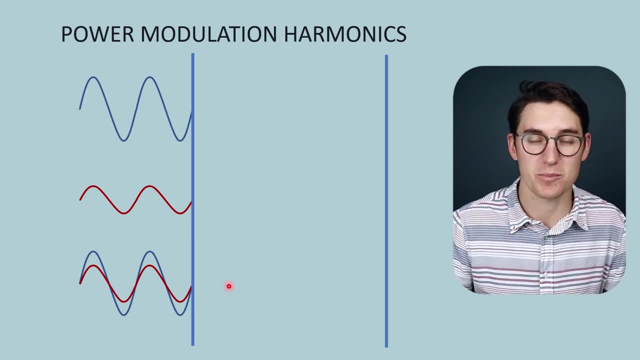 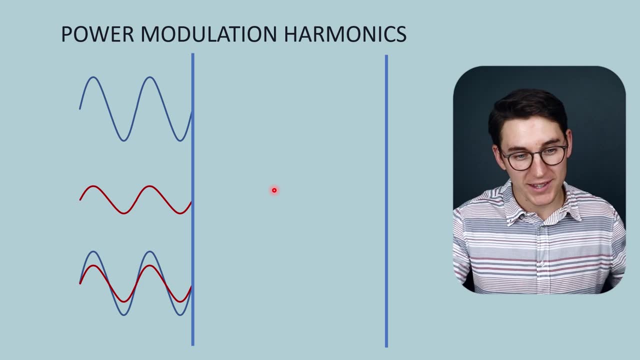 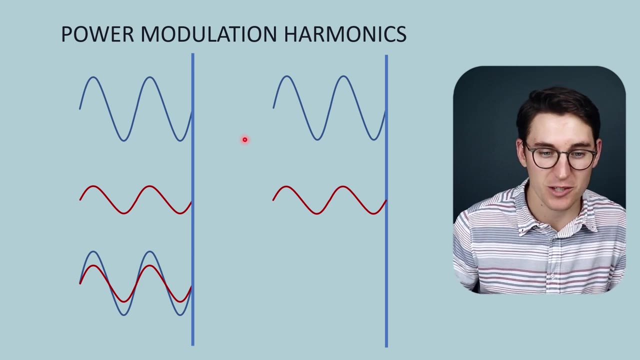 they are going to echo back a fundamental frequency. here we see they don't cancel one another out. now, as we've discussed multiple times now, only regions of high intensity will create a harmonic frequency heading back. so when these ultrasound pulses reach a Slightly deeper tissue of the nonlinear behavior of this ultrasound pulse and the high intensity of this ultrasound pulse, 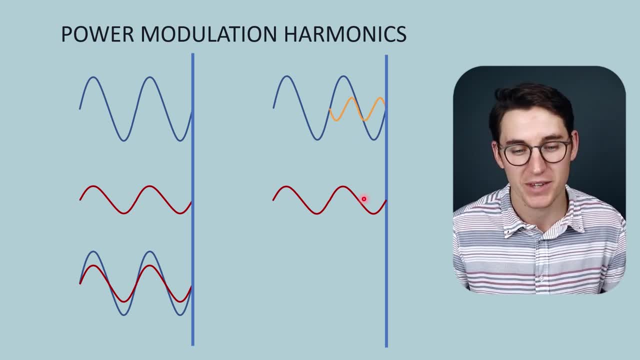 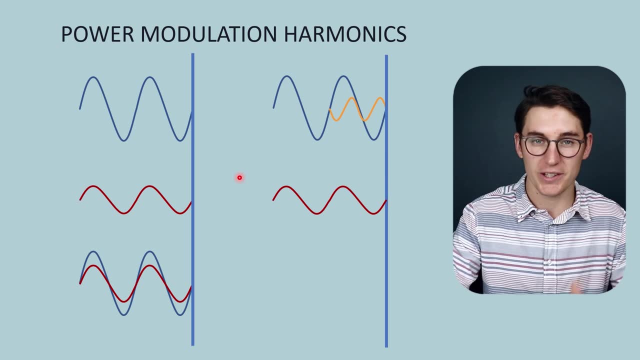 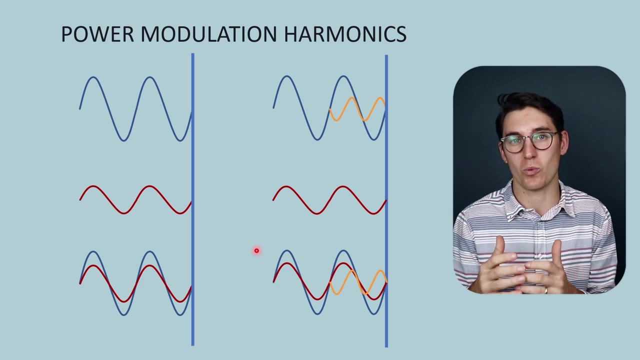 there will be a harmonic created at this tissue boundary. This second ultrasound pulse doesn't have enough intensity to create that tissue harmonic Again. we'll get those returning back to the ultrasound transducer. Now the ultrasound transducer is not seeing these waves as separate. 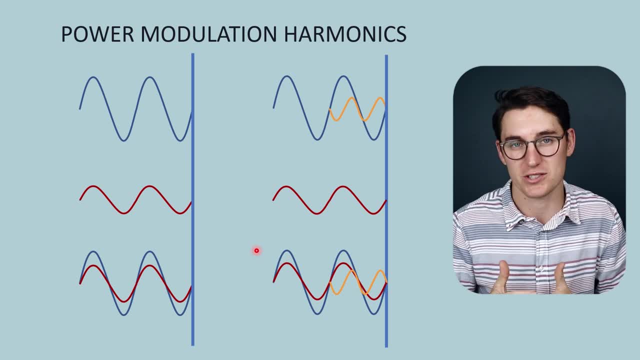 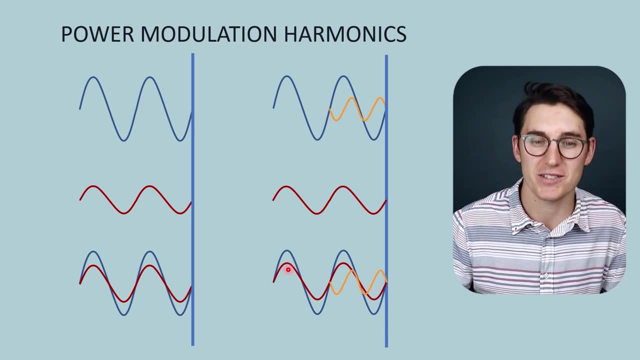 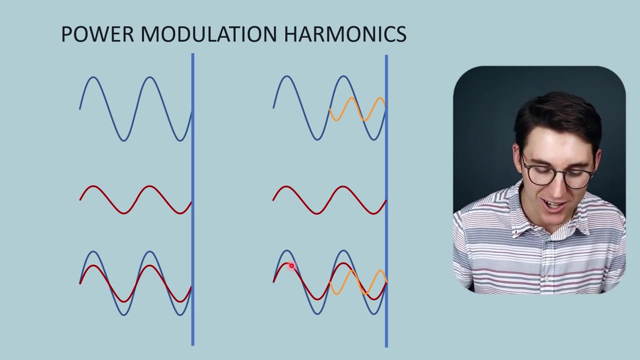 waves, it's getting a combination of that wave coming back towards the ultrasound transducer and, because of the differing amplitudes but same frequencies of the red and the blue waves here are fundamental frequency waves heading back, the ultrasound transducer can use a Fourier transformation to cancel out the contribution of these two waves, cancel out the contribution of. 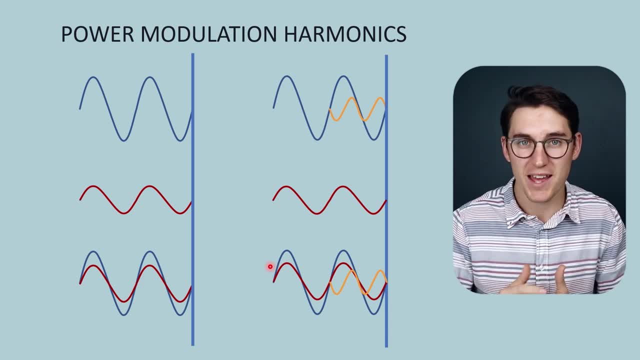 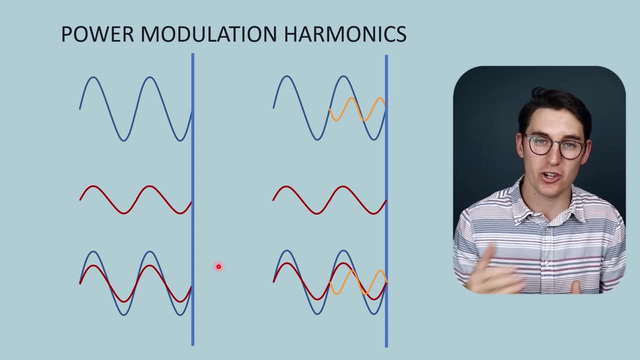 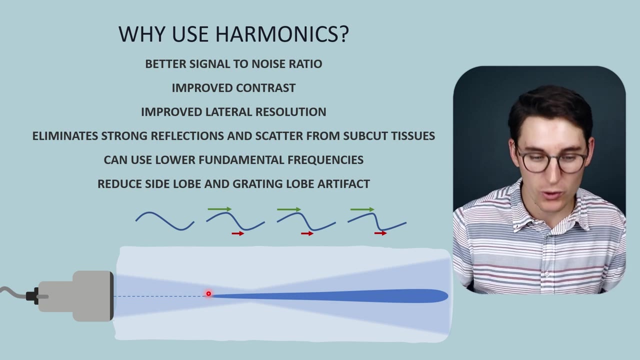 the fundamental frequencies heading back to the ultrasound transducer. That mathematical cancellation will allow the ultrasound transducer to calculate the harmonic frequency that is returning to the ultrasound transducer. Now why do we use harmonic frequencies? We've said that harmonic frequencies only happen at intense 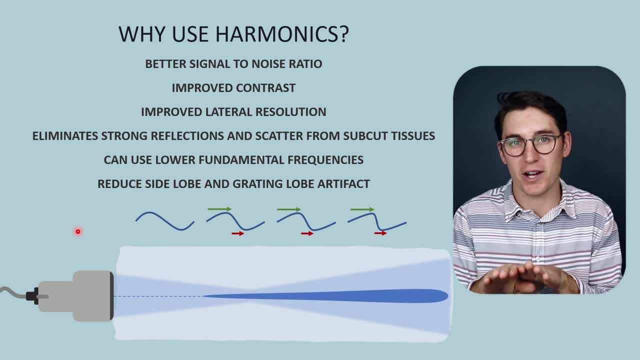 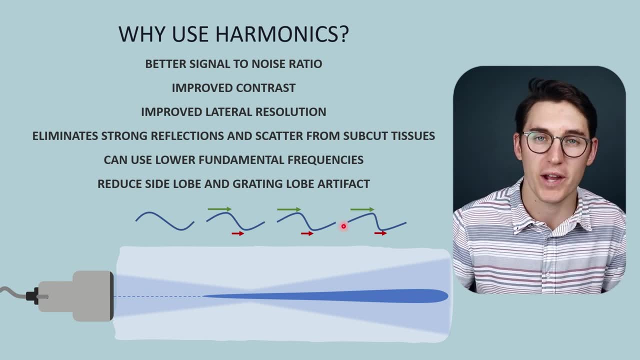 regions of the beam and they only happen at true tissue boundaries. It's the tissue that is creating the returning harmonic frequency based on this nonlinear behavior of the wave propagating through tissues. That gives us better signal to noise ratio: The noise or the scatter that's coming. 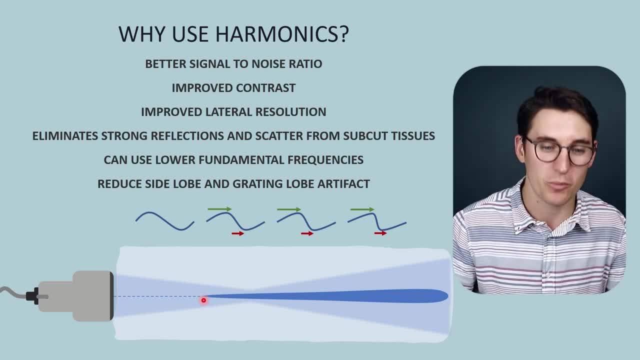 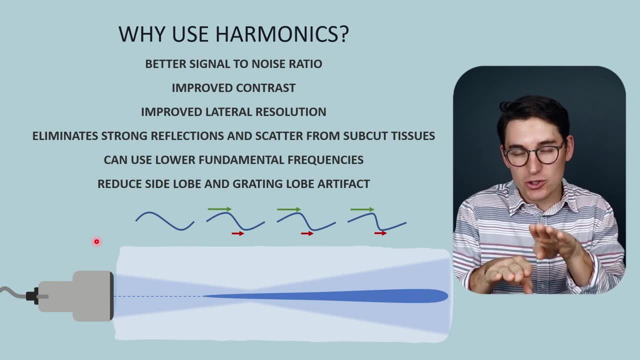 back from our fundamental wave is not contributing to those harmonic frequencies. We are canceling those out when creating the harmonic frequency. So we're not creating the harmonic frequency, but we're creating our beam mode image. It also gives us better contrast. We're getting true contrast. 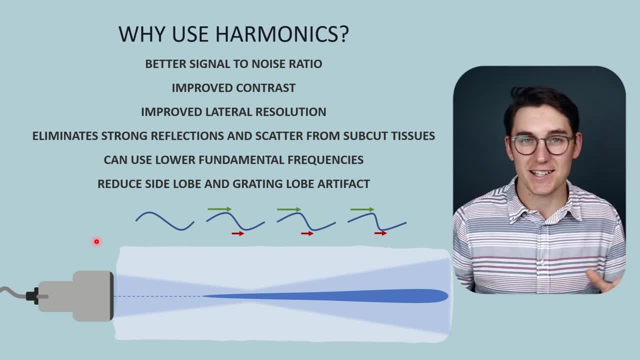 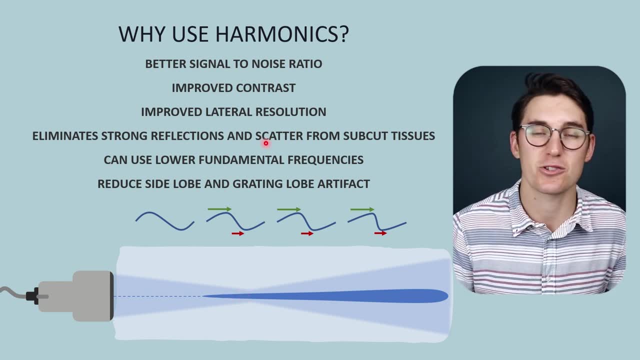 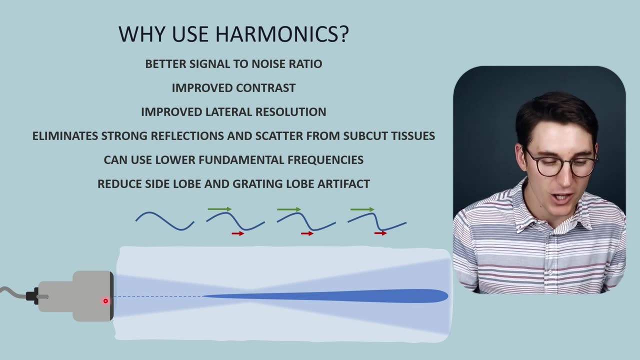 between the tissue boundaries, as well as reducing the scatter and noise that degrade contrast within our image. Because this intense part of the beam is narrower than our actual beam, we get better lateral resolution and we're eliminating the scatter and the reflections that are happening in the subcutaneous tissue. here We've seen that the fundamental frequency heading out into tissue 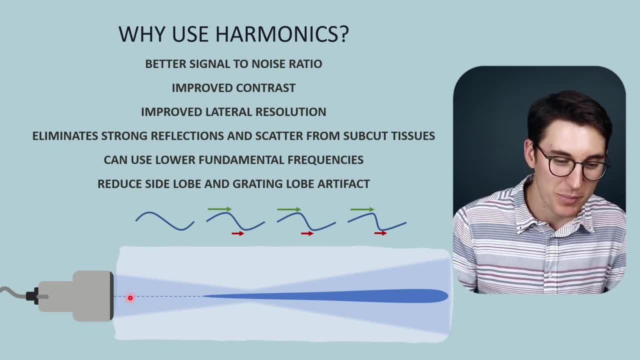 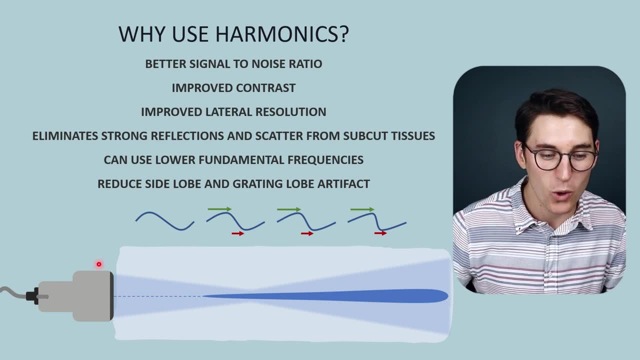 attenuates over time and we get really intense echoes coming back to the beam mode image. We're getting really intense echoes coming back close to the ultrasound transducer because the wave's intensity that we're heading out into the tissue is extremely high. here We can cancel out those. 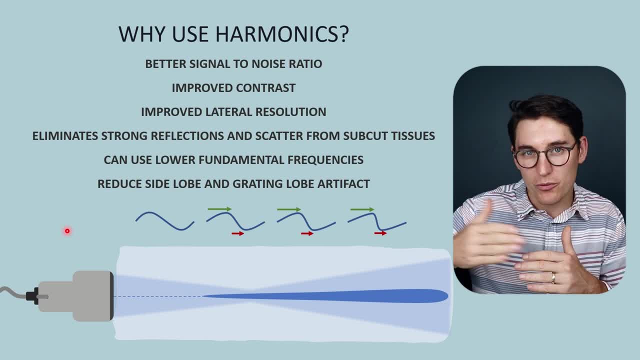 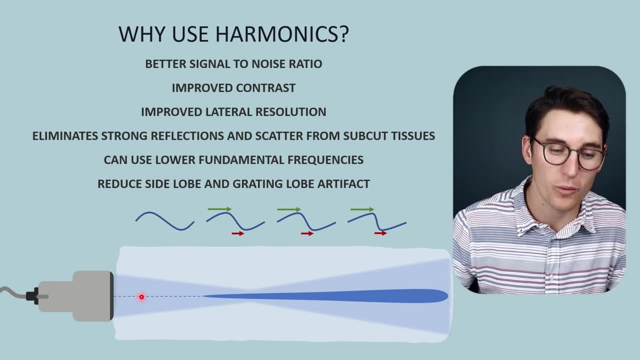 intense waves heading back at the fundamental frequency and the reverberation that happens in the subcutaneous tissues and get better resolution. in this near field We only get those small harmonic frequencies heading back, but because the wave is so intense here those small harmonic frequencies can still give us a good image. We can also use lower fundamental frequencies to 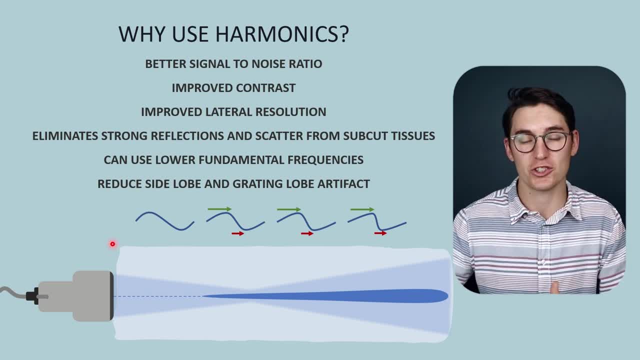 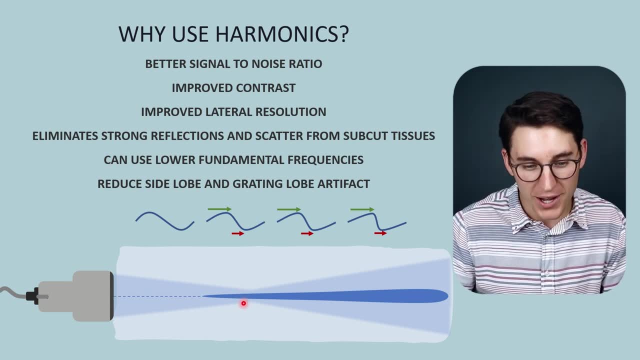 allow us to image deeper into the patient. If we have an obese patient or we want to image deep into the abdomen, we can use a lower fundamental frequency that gets attenuated slower, but get returning harmonic frequencies, higher frequency, returning waves that only have to travel half the 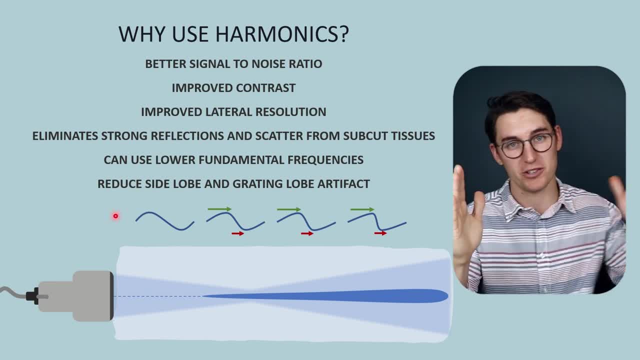 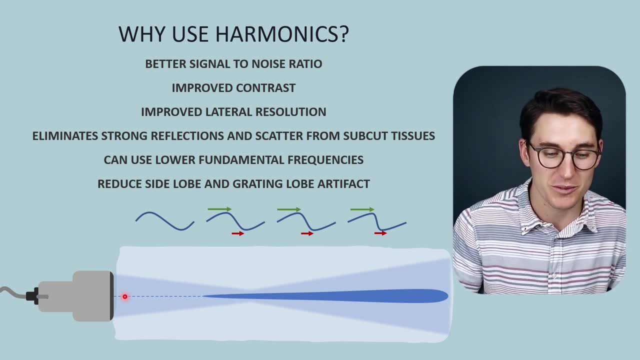 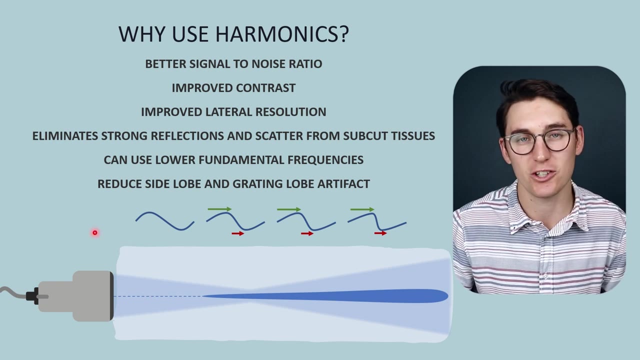 distance. Those higher frequency waves only have to travel from the tissue boundary to the ultrasound transducer. So we get the benefit of receiving high frequency waves, but the depth of the lower frequency fundamental wave that we propagate into the tissue We can also reduce what is known as the side lobes and grating lobes that we've looked at in our 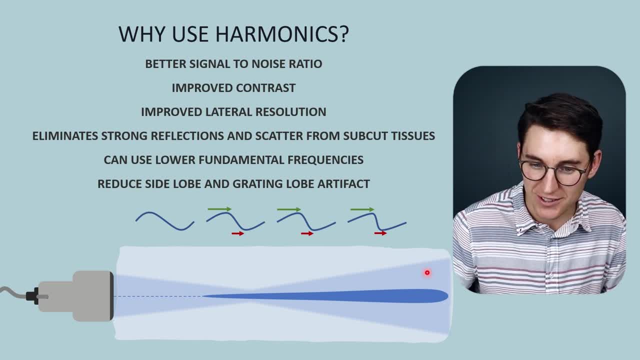 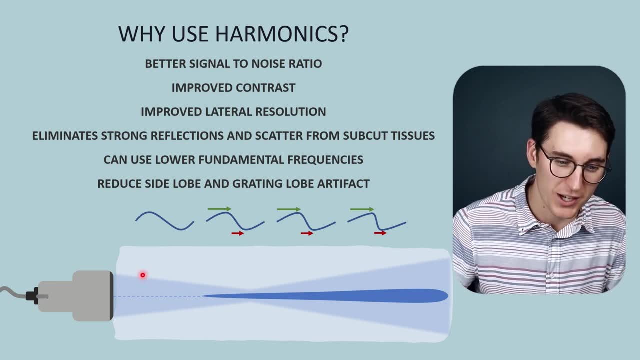 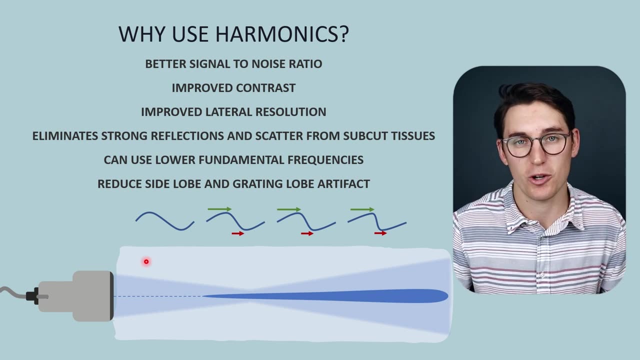 ultrasound beam talk. We saw that when we create an ultrasound beam like this, we get a phenomenon known as side lobes heading out laterally to our beam and grating lobes also heading out lateral to the main ultrasound beam. The intensity of those lobes aren't strong enough to create tissue. 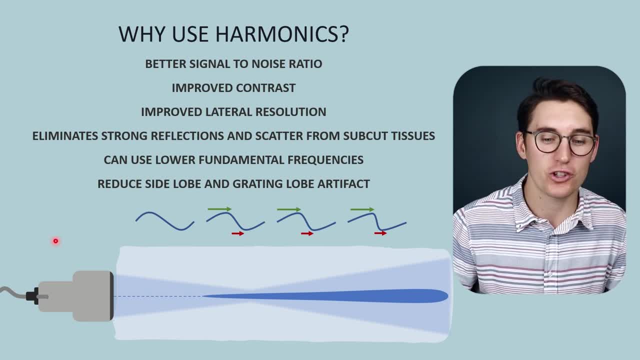 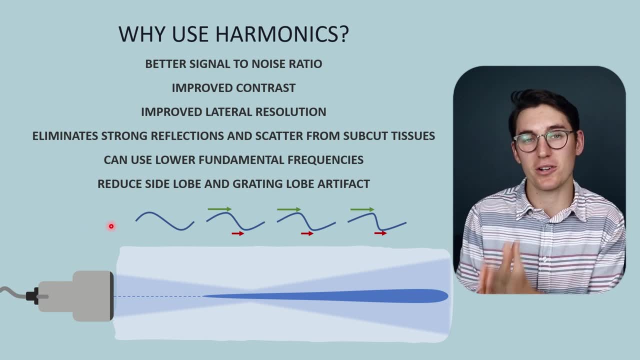 harmonics so we don't get those returning echoes contributing to our ultrasound image. Now harmonic imaging is very important. I'm going to talk about the visual images we're using here. You can see that the is not always perfect. We've seen that if we use pulse inversion. 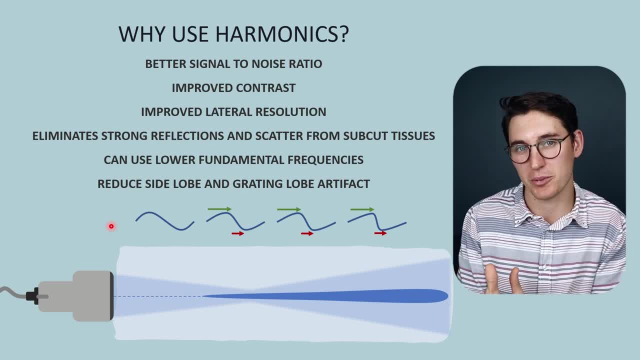 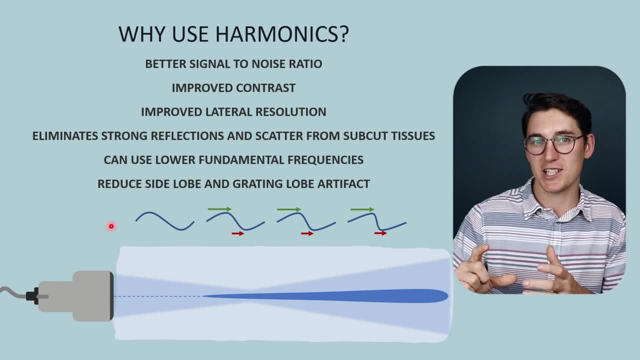 or power modulation modes. we need to send down multiple ultrasound pulses per A-line so we can lose some temporal resolution. Our frame rate will have to slow down ever so slightly. We've also seen that we potentially need to use higher spatial pulse lengths. 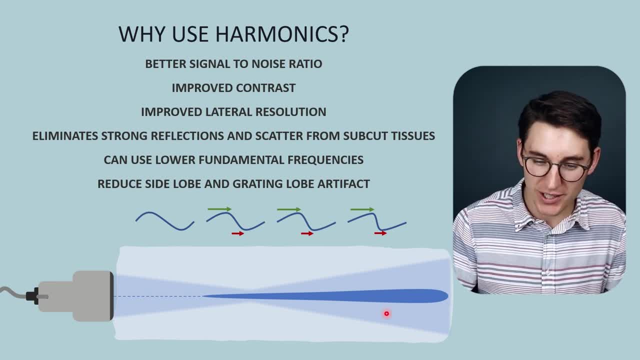 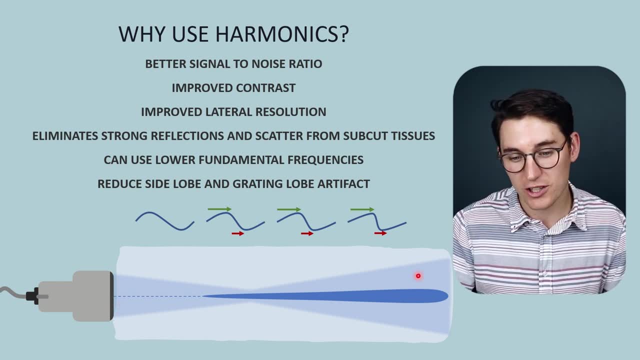 reducing some axial resolution And we've seen that if we're imaging really deep here, the high frequency harmonics aren't going to make it back to our ultrasound transducer. Only those lower, fundamental frequencies will make it back. We might need to use traditional pulse echo ultrasonography. 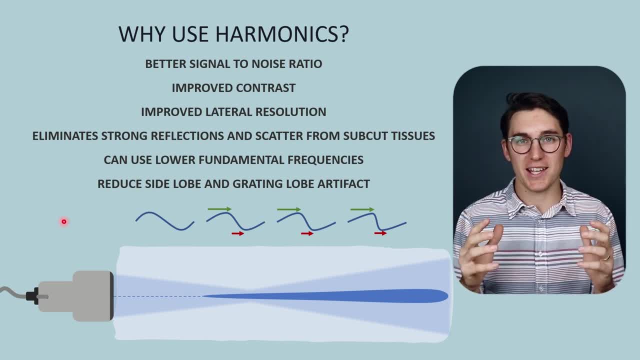 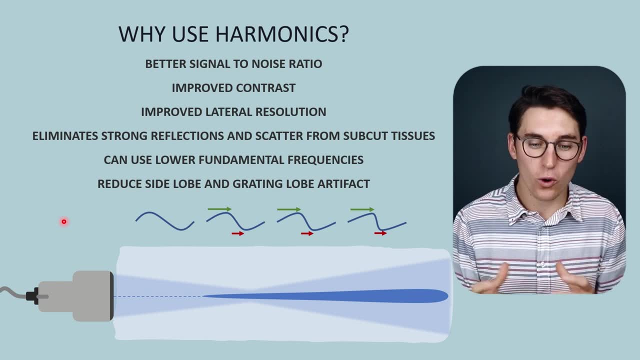 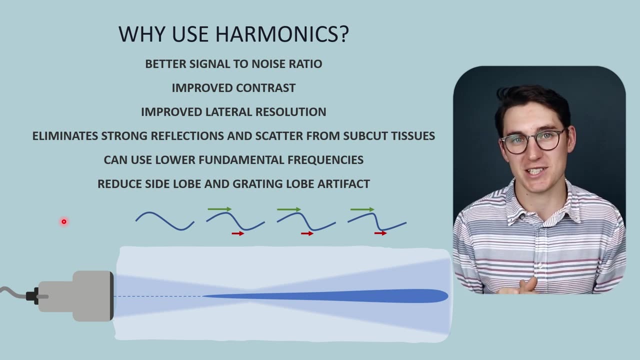 when imaging deeper tissues. Now, harmonic imaging is a difficult concept for people to understand often And I don't want you to get caught up in the core underlying physics here. The core concept here is that harmonic imaging uses tissue harmonics, the integer multiples of our fundamental frequency.